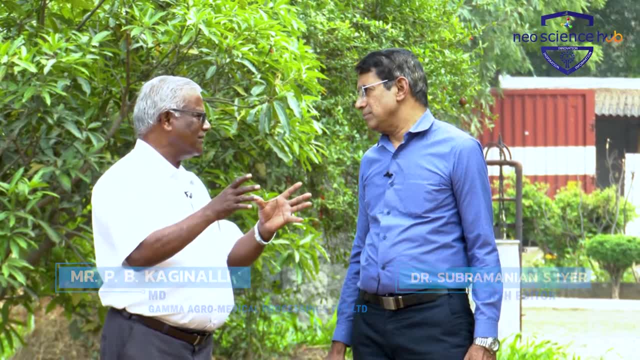 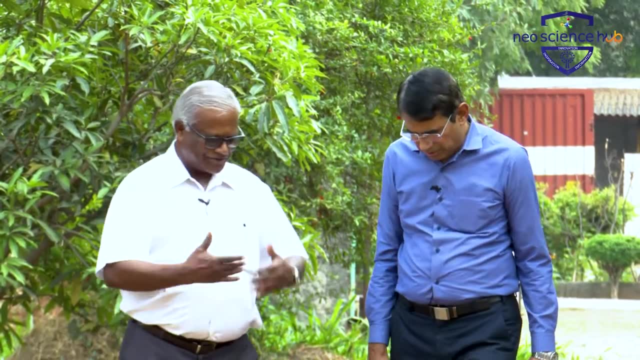 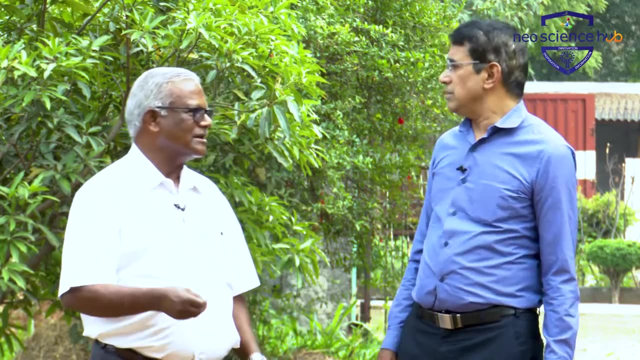 Okay, That is flaw detection in the pipeline, welded joints, pressure vessels- Ok, very good. And then I changed my profession to medical applications of radiation- Ok, Wherein radiation is used to treat cancers- Good, This is my cancer. Yeah, And in that cobalt isotope is also used as a teletherapy- Yes Applications- And further as a. I mean in the tumor bed itself. we can keep the radioisotope. Oh, ok, See the iridium-192 seeds. Ok, And cesium-137 seeds- see tubes- are also used. Ok For ladies cancers like uterine cancer. Ok, And some of the head and neck cancers. Yeah, I mean iridium-192 seeds are used. 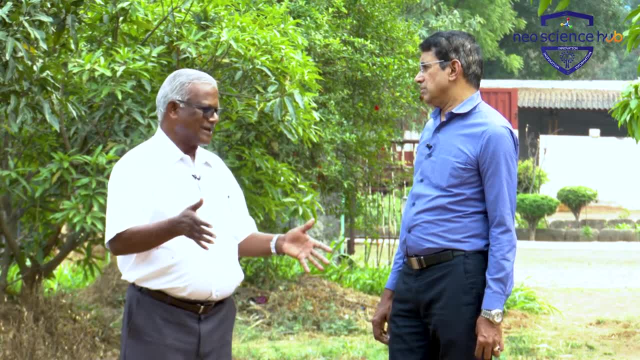 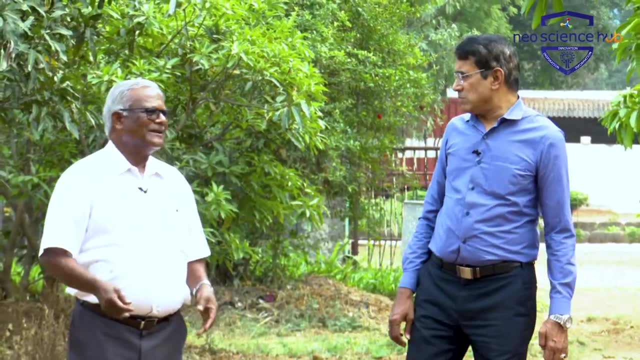 Correct See, of course it was almost I left. I left that field about 23 years back. Ok, Ok, 25 years, 25 years back, huh, Yeah, See, I felt I should do something more. Sure. I spent about 13 years in the medical line. Ok, Some of my appetite. Appetite, Yeah, Appetite for further growth, Further growth. Yeah, It didn't. I was dreaming of, Ok, Ok, See, this project I was dreaming of for almost 20 years. 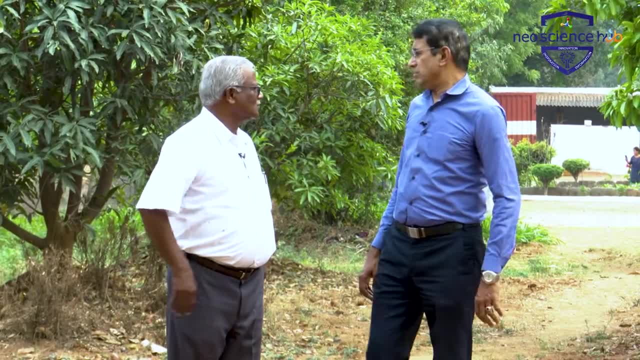 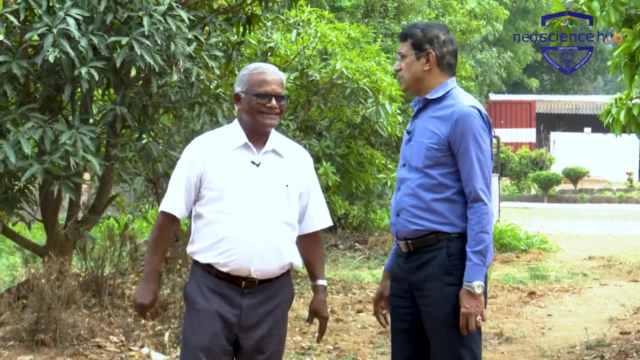 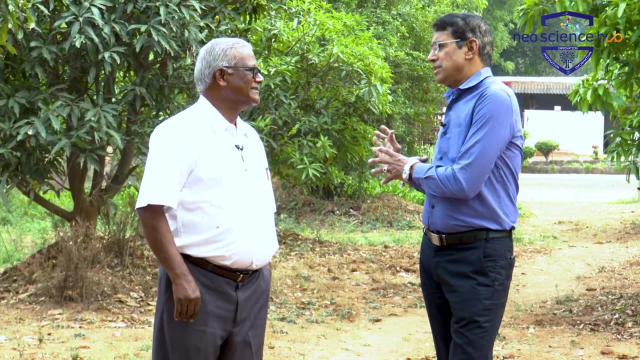 So when was this established? This- This is in 2008- is commissioned, Ok, Ok. Before that, there is a lot of speed work also, Of course. Of course I understand, I understand. Now, how do you ensure that your work in this is supporting the food industry? 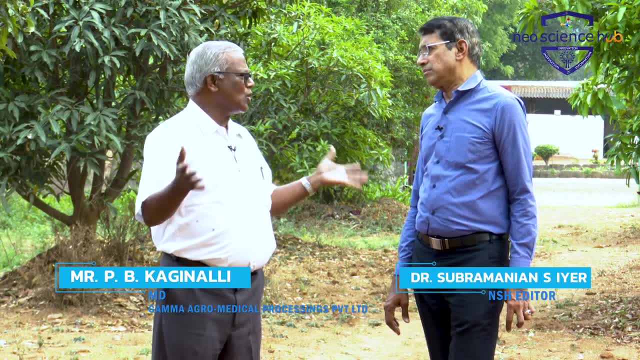 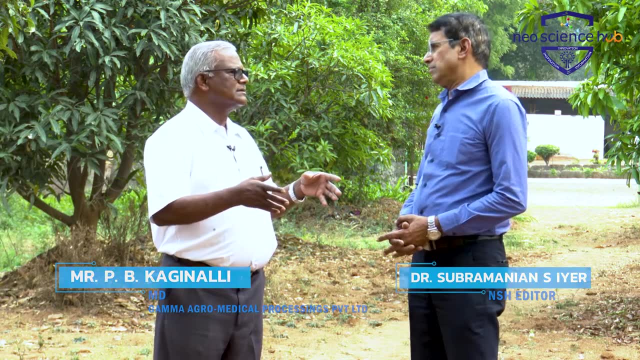 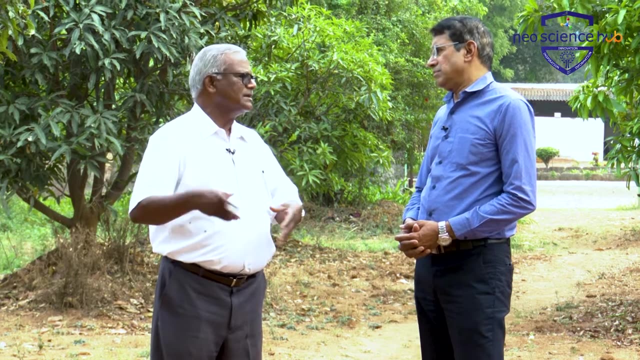 See, lot of food is grown, no doubt Because of handling storage for so many reasons there is a huge spoilage. you know, In the godowns there are leek rats, mice, they eat away And so many. 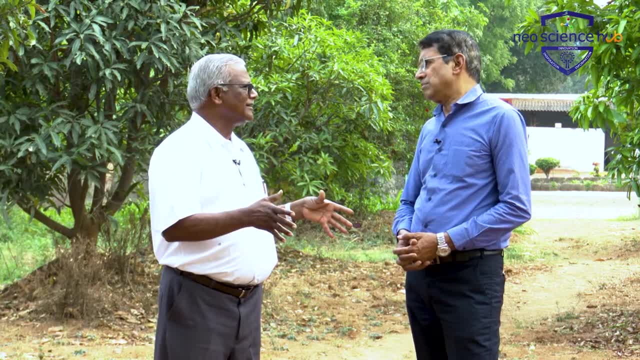 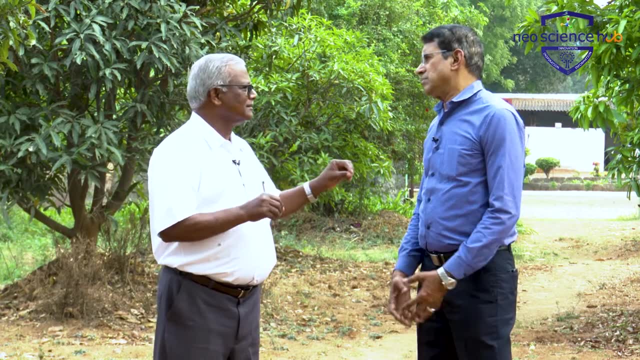 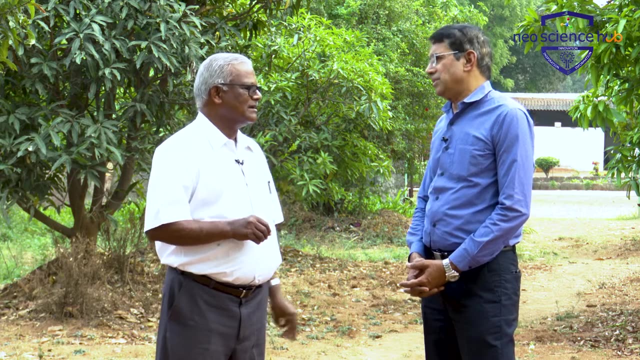 I mean in handling agricultural products. unfortunately we have left the field to totally an uneducated class. Agriculture is not a propagation of this thing. Professionals are educated class. I know. I know Only because drudgery involved Hard work. 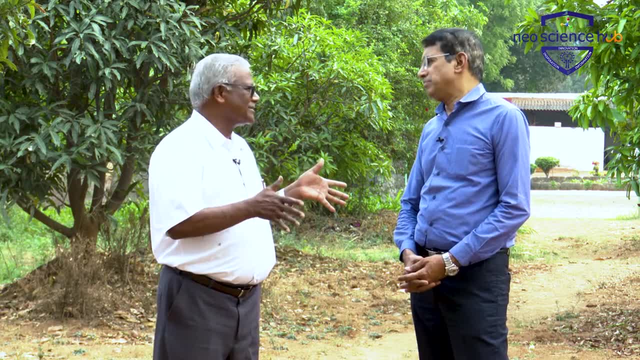 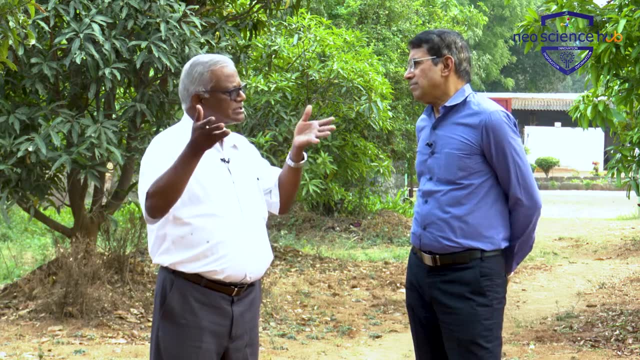 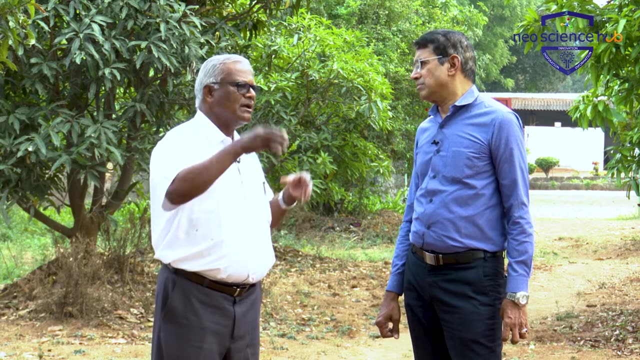 Hard work involved. Mining is working involved. See, nobody prefers agriculture, no doubt about it, Correct. And that way, handling there. of course, some traditional knowledge is there, But we need some educated people to handle the product, to grow the product, plants requirement: 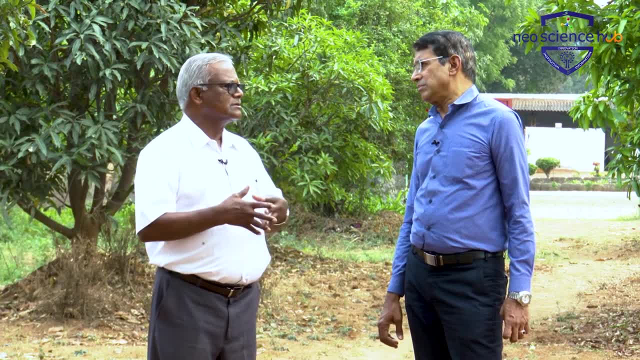 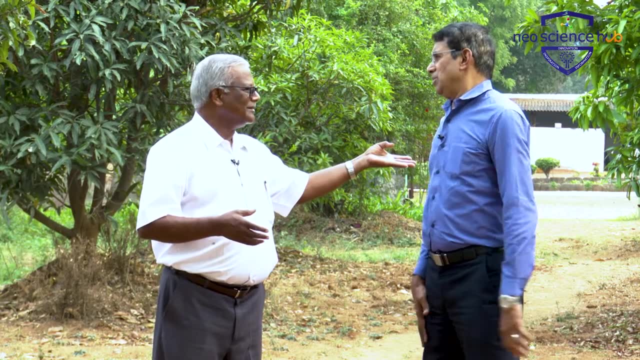 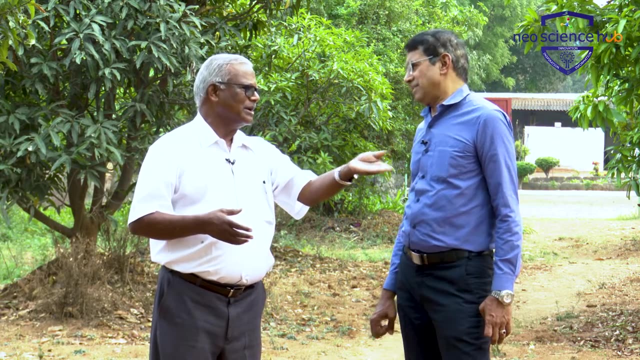 I don't know And I am very sorry to see the things that people- engineers- like they are working on non-living items. I know Absolutely Like metals. Correct, Mostly metals and other materials. Yes, Non-living materials. 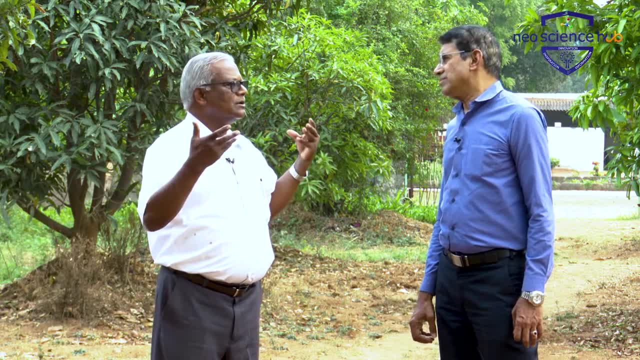 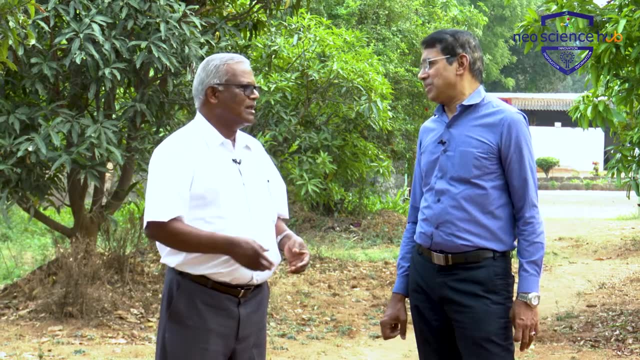 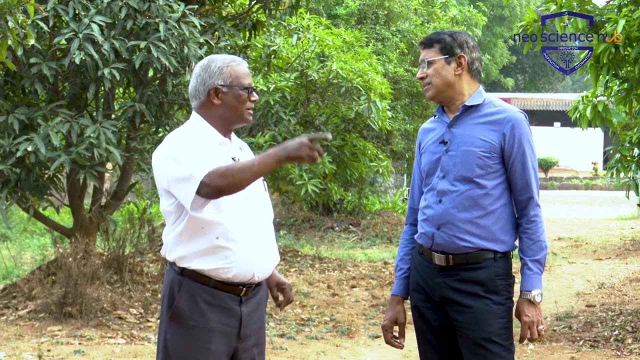 Yes, Non-living, yeah, And their skill is, I mean, exaggerated, and they say… High, High, High. this thing is given to them, Correct, Whereas this is a living plant. Absolutely, Absolutely. This needs absolute study, because anything goes wrong. you are going to have the effect. 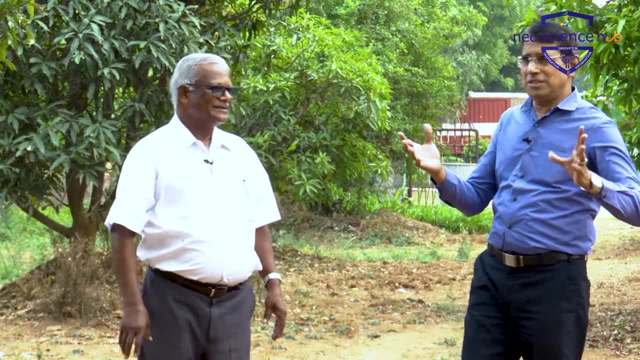 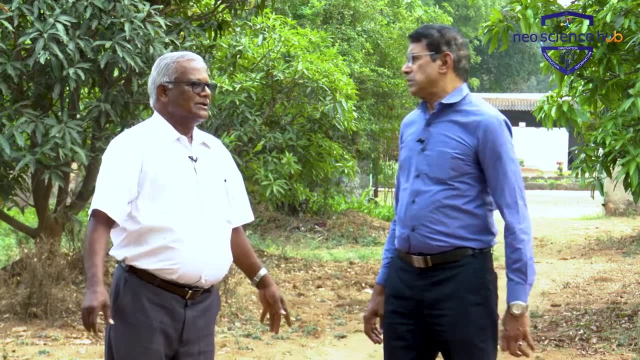 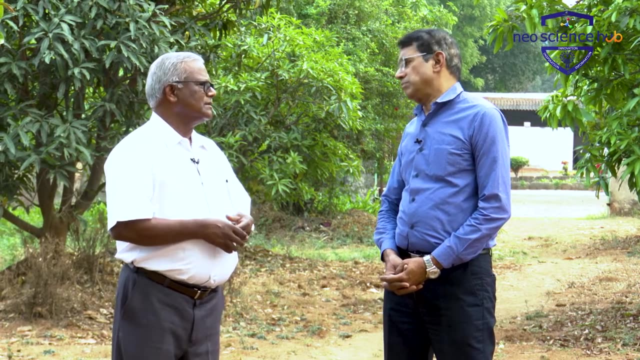 of it. I can see the passion. I can see greenery all around. Now you have to tell our viewers what you are actually doing in this organization. See, we are processing food products like spices, herbal extracts, pet food and spices. 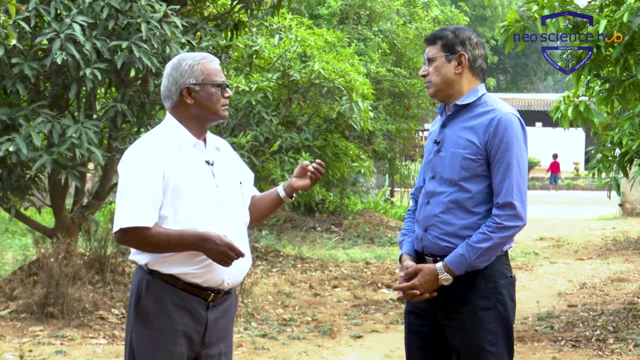 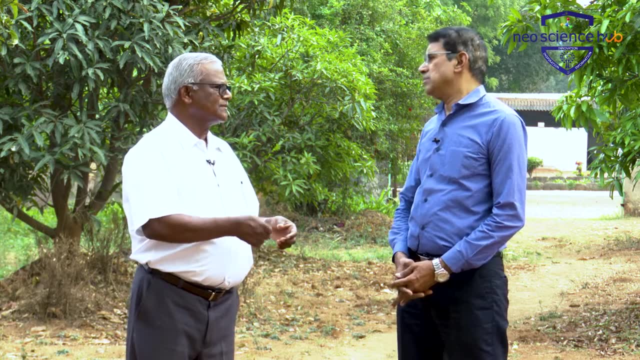 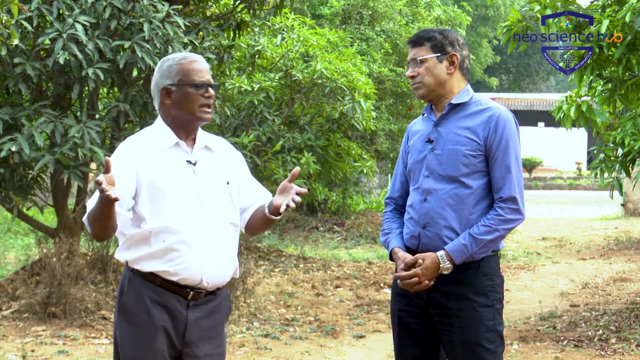 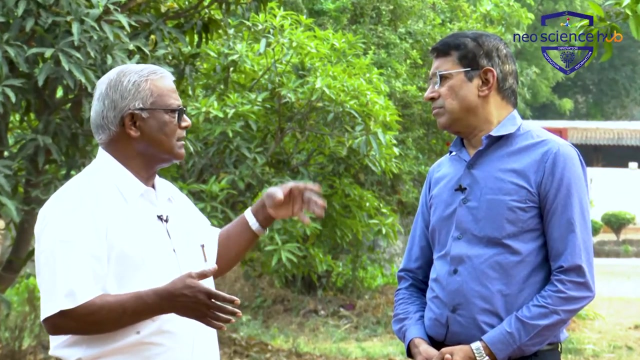 like chili powder And medical products like vaccine containers, packaging material: mainly Sure And their flip-off seals and some of the lab… See, they conduct studies on lab animals. so clinical trials of lab animals They need. I mean food and bedding. 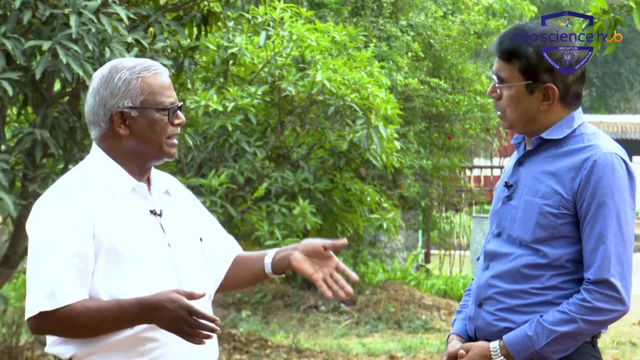 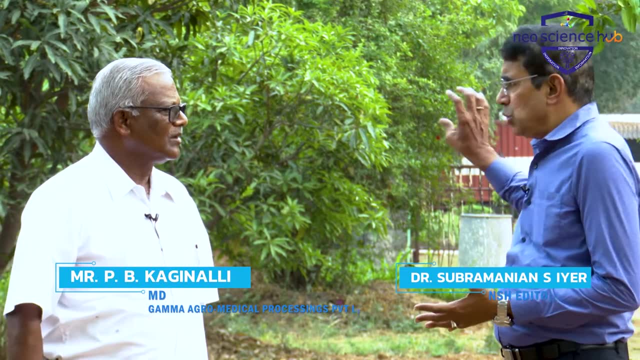 Yes, Yes, Food also needs to be sterile, bedding also needs to be sterile, and their water and all they make sterile. So, in short, all these items come into your organization, into your company… Yeah, …to get themselves sterilized. 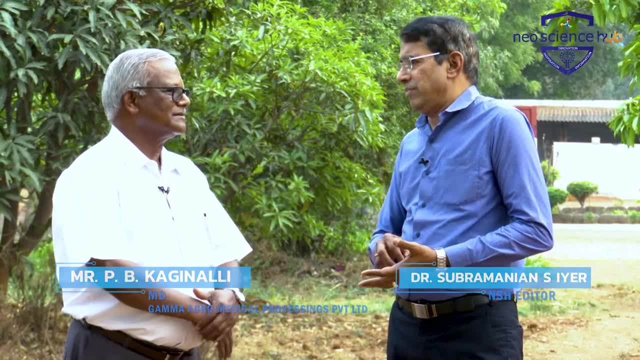 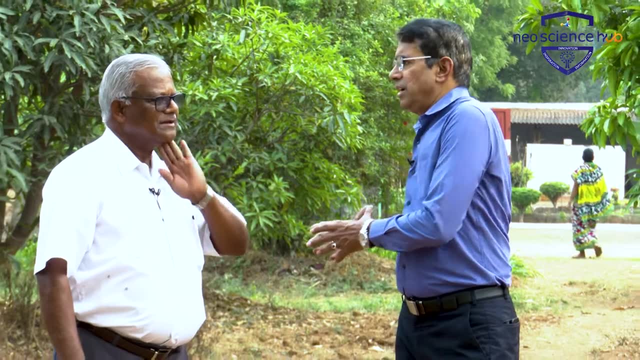 Yeah, Am I right? Yeah, Yeah, Very much For gamma sterilization. Yes, Yes, Yes, Okay, Now this gamma sterilization, how is it vis-a-vis other types of sterilization Like heat, Dry heat? 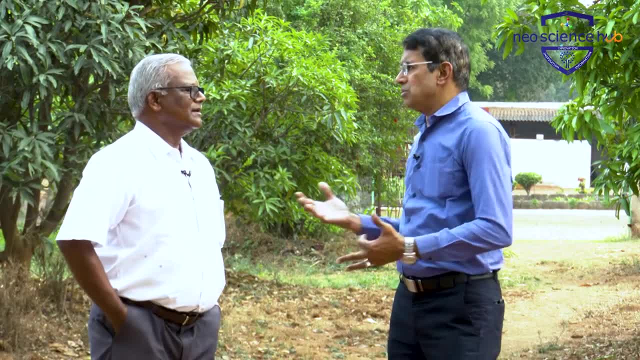 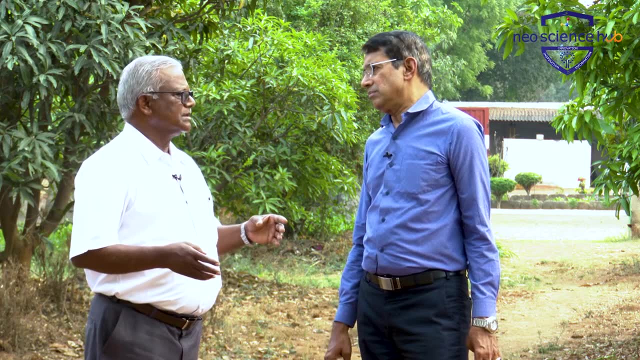 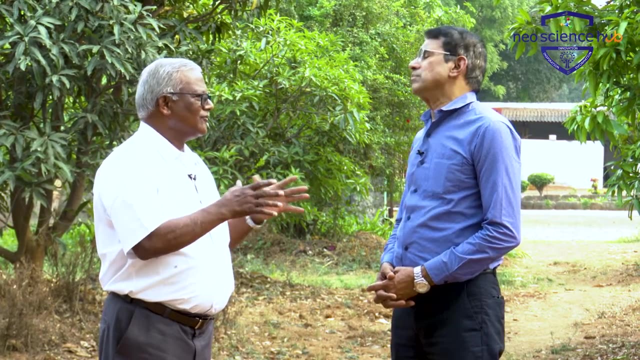 Yeah, Or ethylene oxide, Or gas plasma, How all this… See, you know heat. see, as for food is concerned, Yeah, Heat, Heat. There are certain loss of flavors, vitamins, essential these things, stuff contained in. 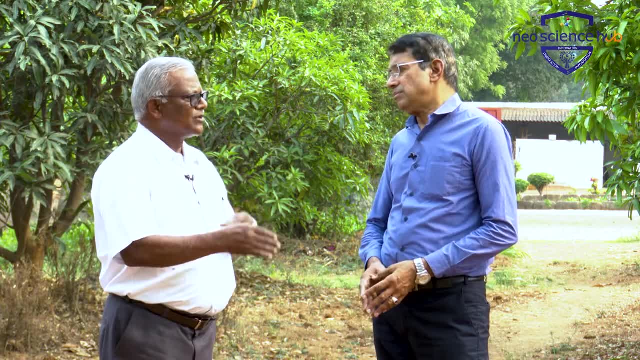 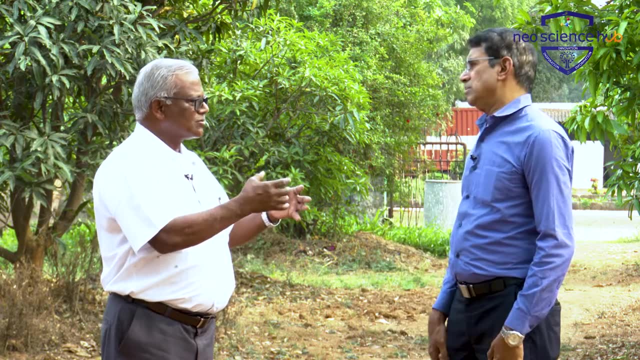 that Yes, Okay, Because of heat. Okay, And further, ethylene oxide is a deadly chemical. It's a poisonous chemical, Absolutely, If it is not thoroughly… Removed …it is impossible to remove, Impossible to remove, Okay. 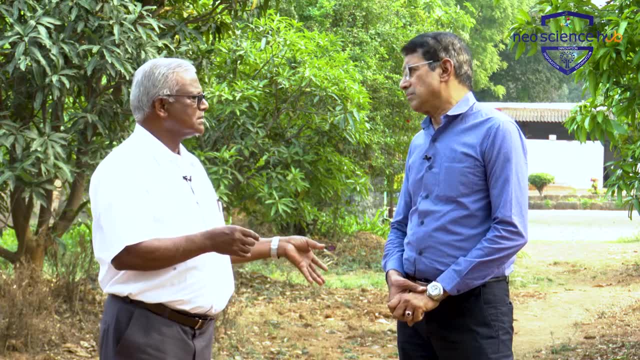 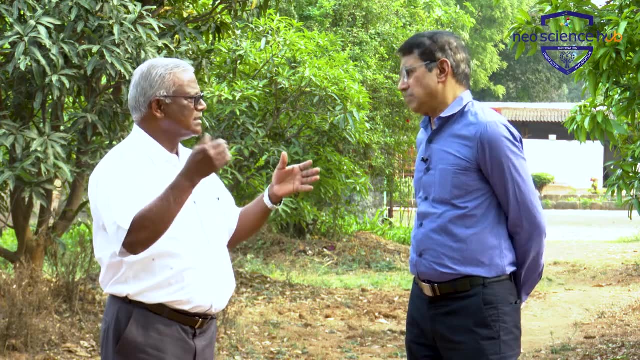 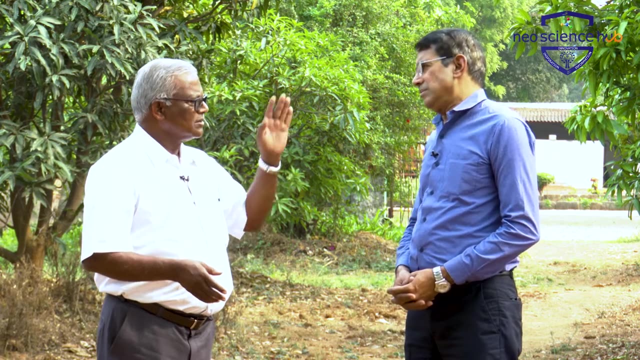 But whatever retained ethylene oxide in the food or medical products, that is hazardous to humans. Okay, There are instances like I mean hemolysis, thrombosis, Correct. There are many issues crop up because of ethylene. It is almost banned in the whole world. Okay, But unfortunately sufficient infrastructure is not available. with alternative technologies, Okay, That's how ethylene oxide is still surviving, Still going on, Okay. And gamma sterilization: in the recent past it has emerged as an alternative. Okay. 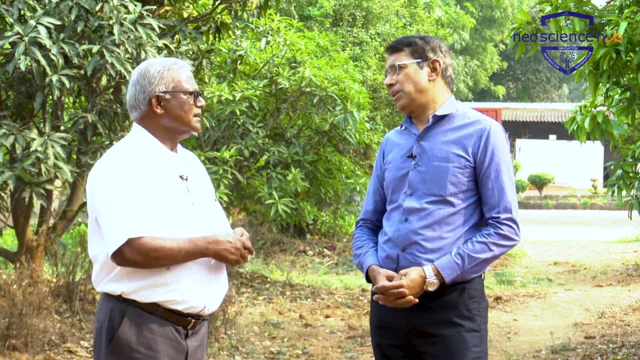 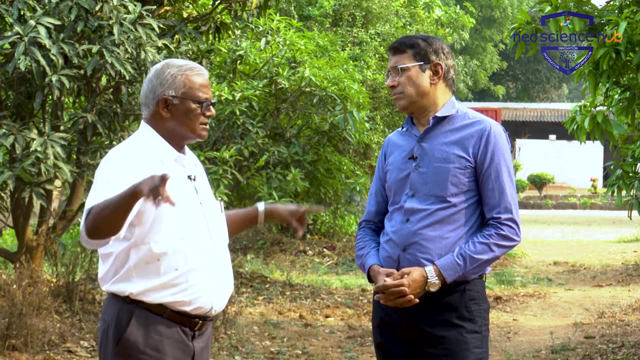 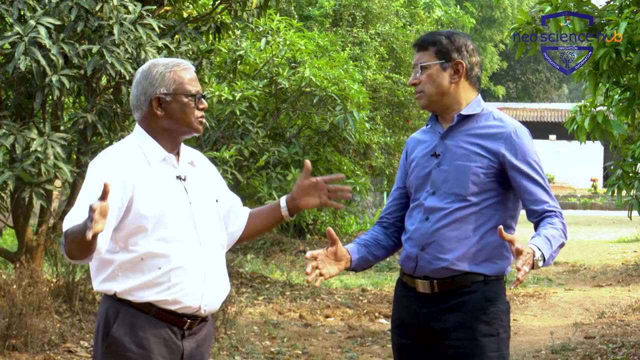 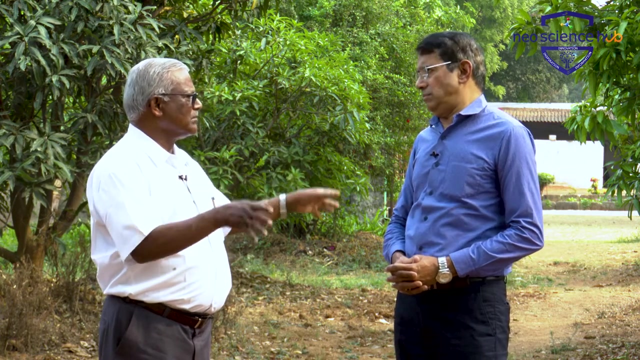 To certain extent to ethylene oxide. Okay, Okay, Because it doesn't leave any residue in the product. At the same time, once the isotope is shielded in a… I mean thick walls, Okay, Walls, Yeah- And it doesn't pose any hazard to the neighborhood or public at large or operators in the facility. 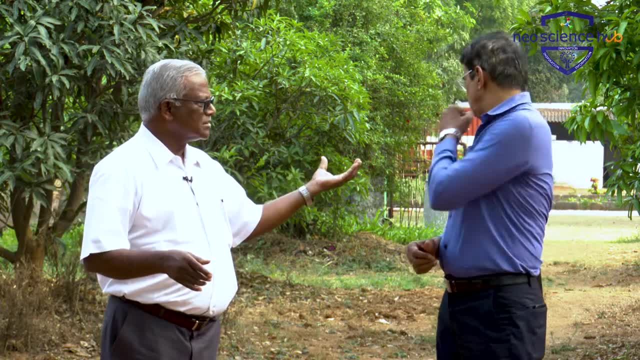 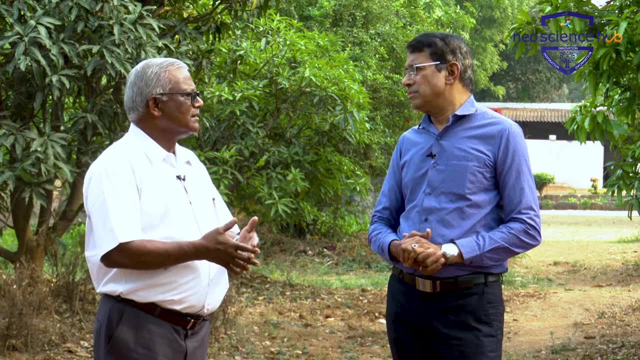 Okay, It is…. I mean, there are no emissions of either gaseous or liquid. Okay, It doesn't generate any waste, Okay, Okay, See, that way. see, it can be an eco-friendly alternative for any other…. 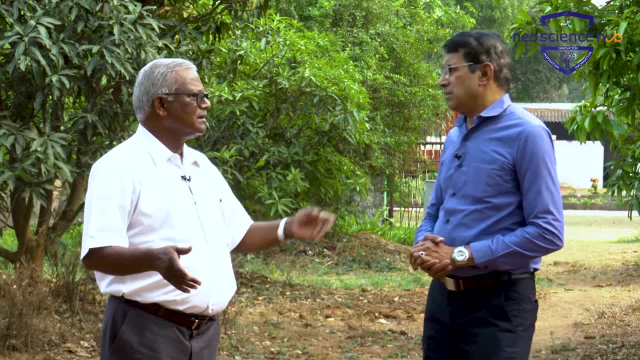 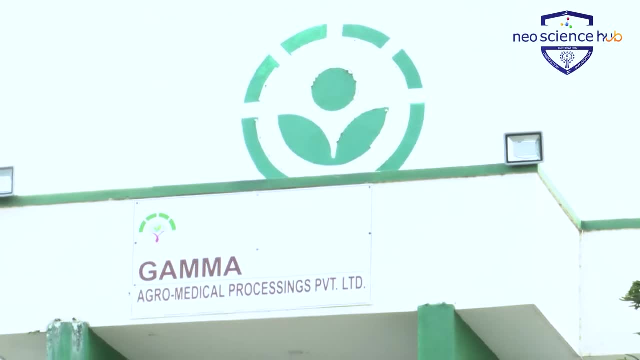 Fantastic, Fantastic Either. if you want heat, you have to burn coal or electricity. Lovely, Very few people know about this. Yeah, Okay, What is the theory behind gamma radiation? You have told me what you do, but I just want my viewers also to know. 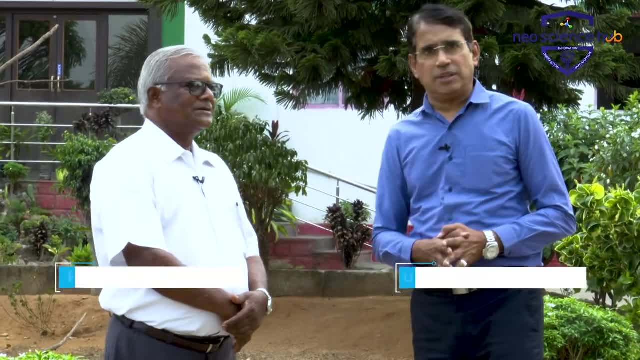 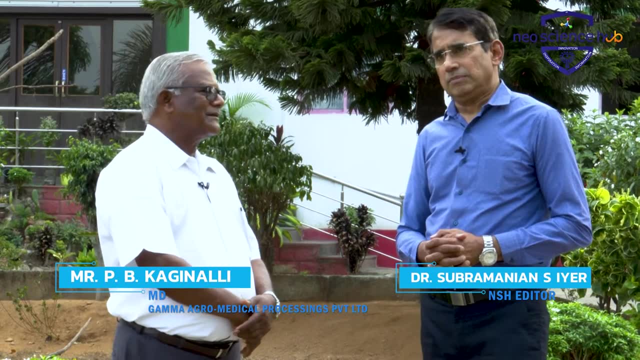 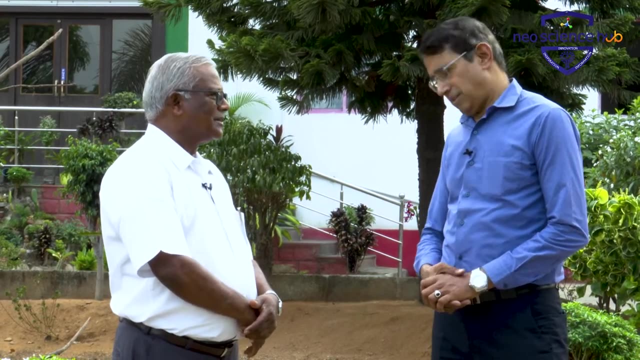 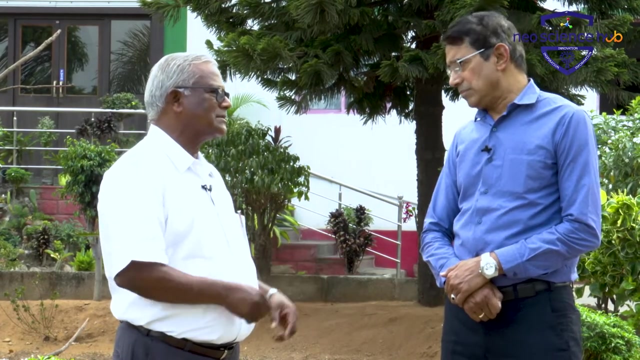 The theory behind the gamma radiation. See, you know, in the nuclear physics…. Yeah, Atom contains electrons revolving around the nucleus. Okay, Nucleus has got protons and neutrons in it, Correct? And because of certain natural imbalances in the nucleus, they are vulnerable for fission. 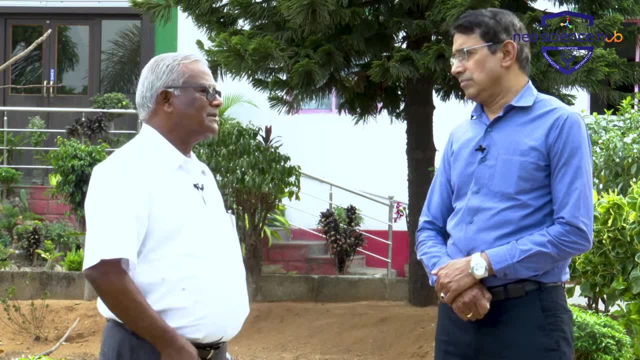 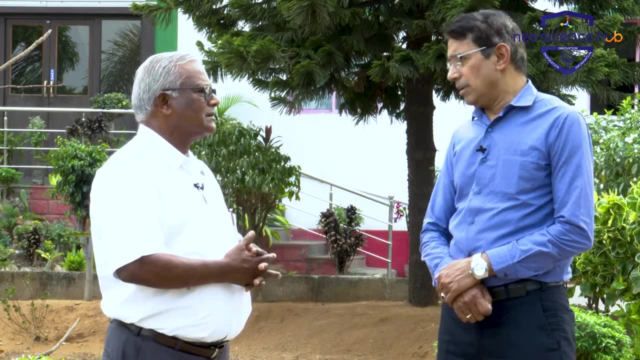 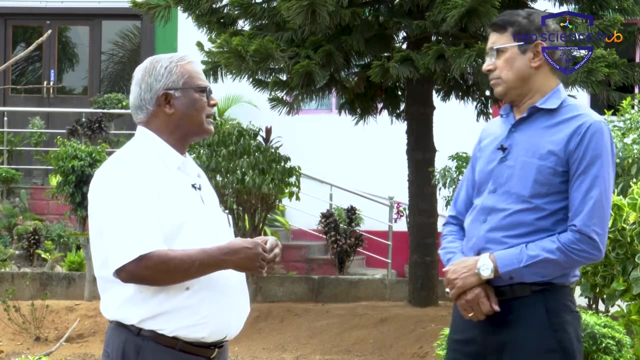 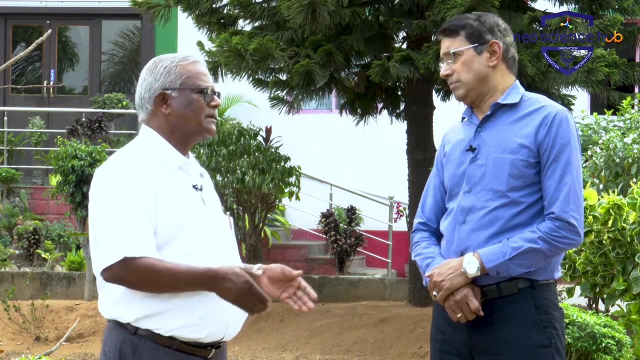 breakup or emissions: See. sometimes they are naturally existent, like potassium-40, and uranium thorium. These are there naturally, which are of high atomic number- See. instant fission is also possible. They break up instantaneously. 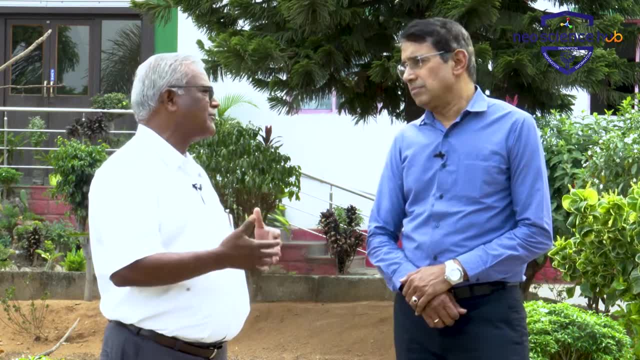 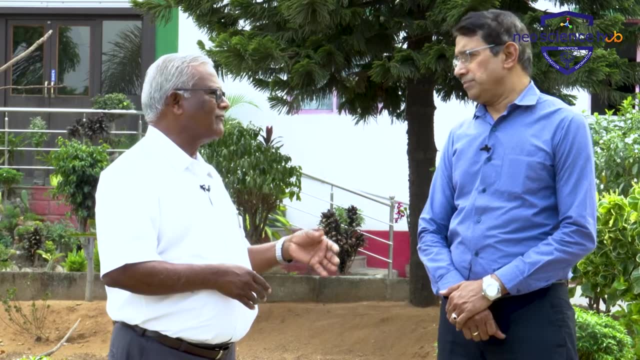 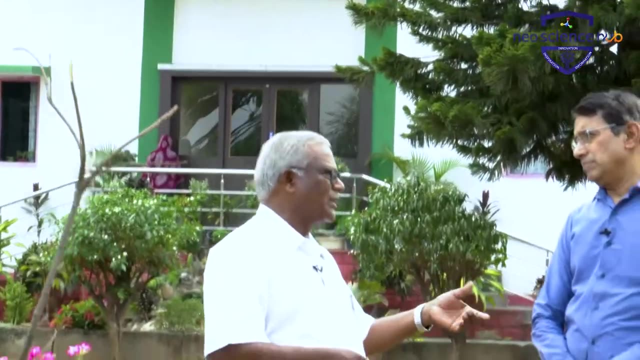 There are certain particles which emerge from the nucleus in this process of… Absolutely …break, Yeah, Say alpha… Fission, yeah …alpha, beta and gamma Gamma, Alpha, beta are charged particles. Alpha is nothing but helium nucleus. 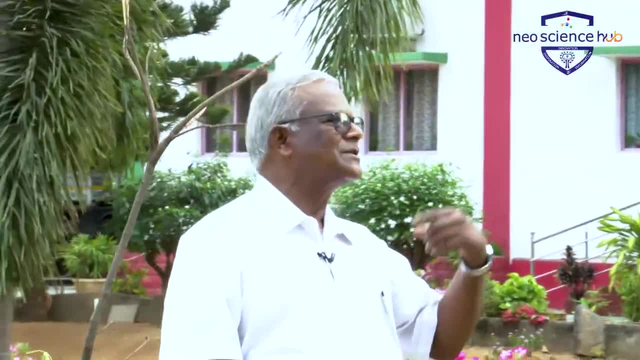 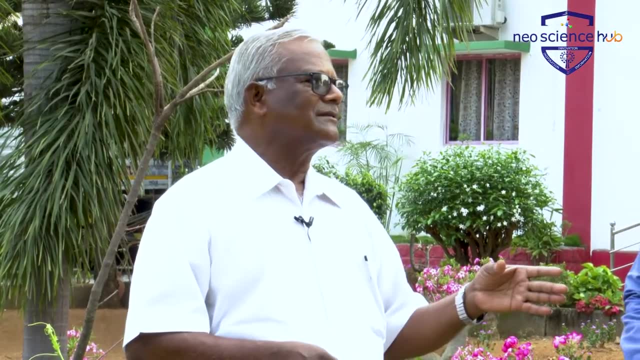 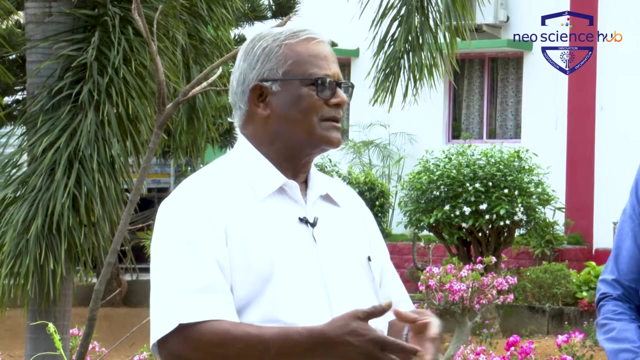 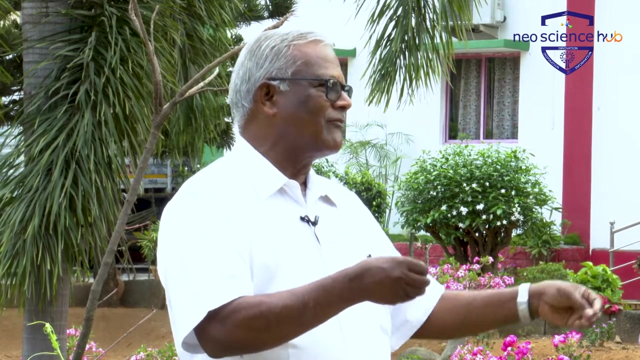 Okay, So once it becomes…it gets emitted, it becomes helium atom. Right, Beta is an electron…nothing but an electron. so that gets, I mean, interacted with matter around it in the air. Okay, And gamma… So gamma is the one which, due to energy left behind by either alpha decay or beta decay, 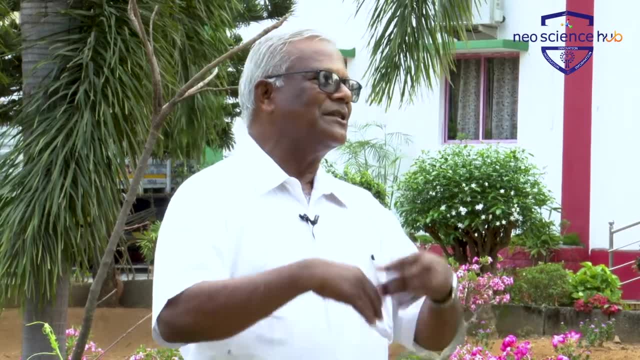 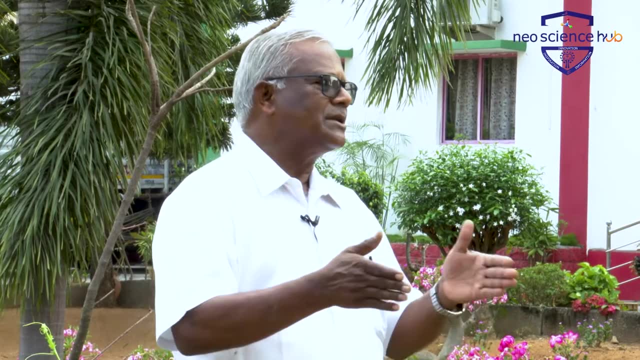 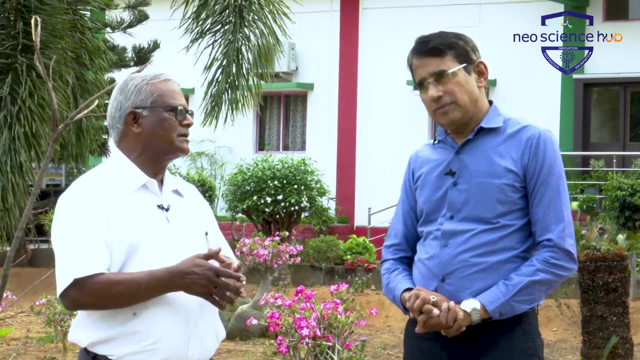 the left out. energy is emitted in the form of gamma radiation, So it has high penetration. Yes, gamma radiation has got high penetration. I mean it is a non-charged particle, So it has got ionizing characters as well as high penetrating power also. 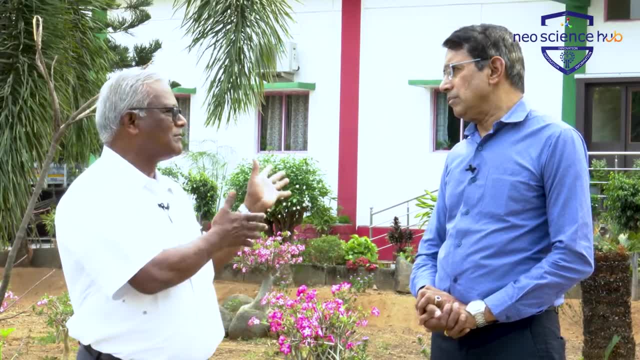 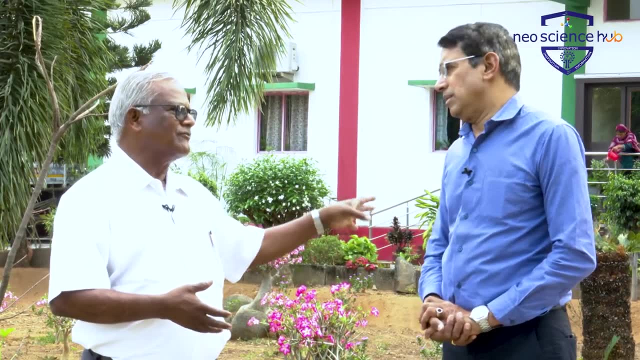 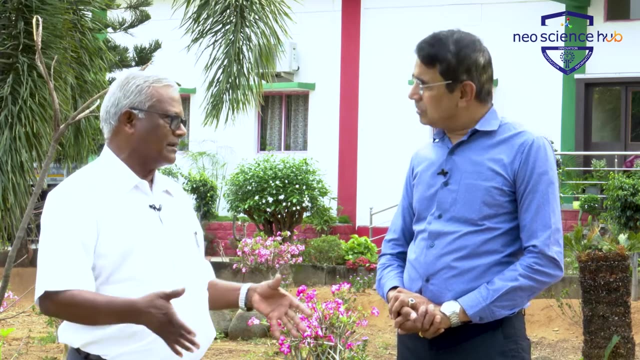 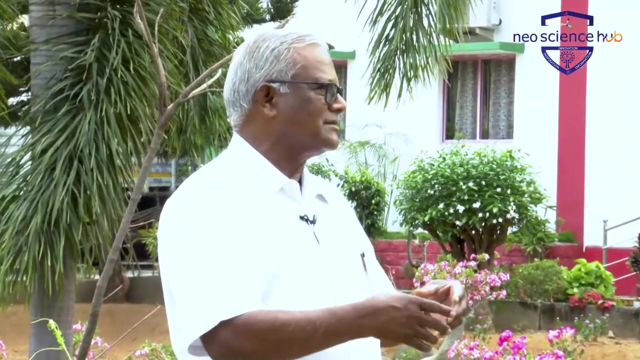 Because of high penetrating power, see, we could use them for a bulk of agricultural products for treatment of disinfestation and microbial decontamination. And another characteristic of gamma is it ionizes the air, or any product for that matter. See, this ionization is utilized- its characteristics are tapped- for processing the food. 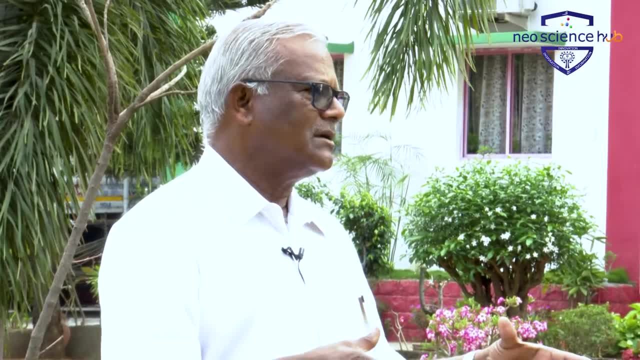 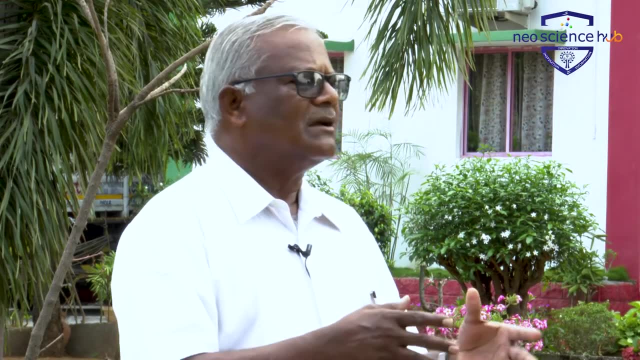 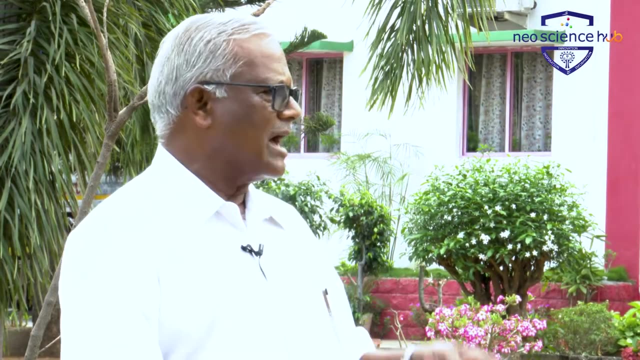 Ok, So only food is dry one and it does not have any living stuff in it. Ok, After grinding or this thing, It kills all the bacteria, kills all the microbes. See, whichever bacteria or insects, pests are present in the product. 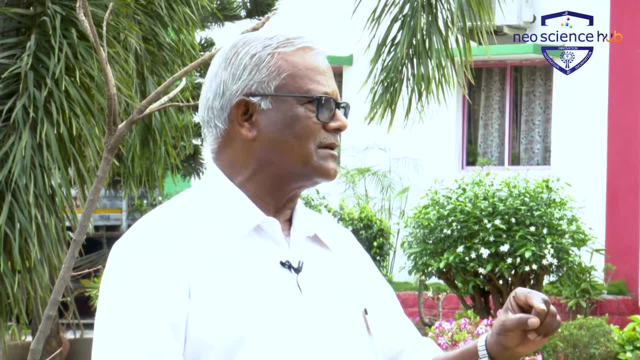 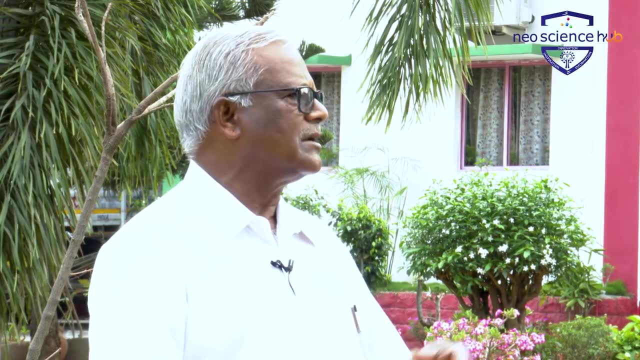 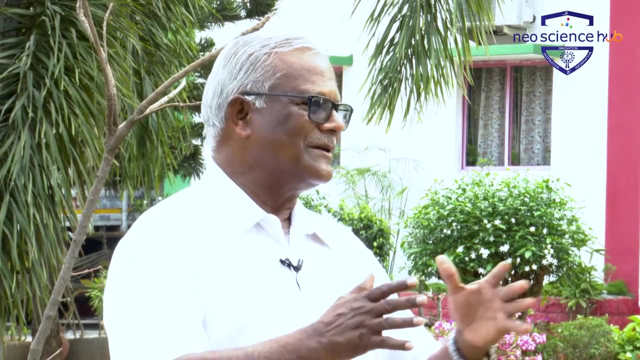 See water. hydrolysis of water is one thing, radiolysis of water. See in that process what happens? Hydroxide and hydroxy radicals are formed. Ok, See, these radicals are very dangerous. Correct, They in the living organism. they break, interact with the DNA chain and break the DNA chain. 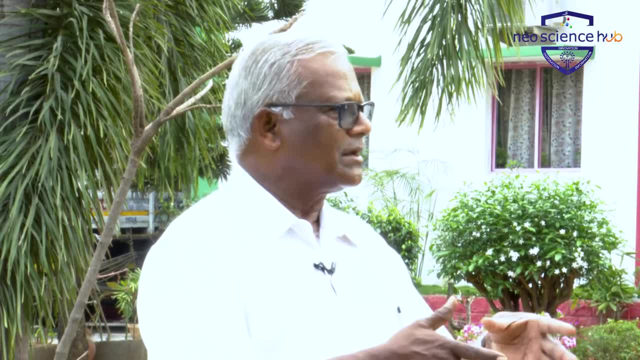 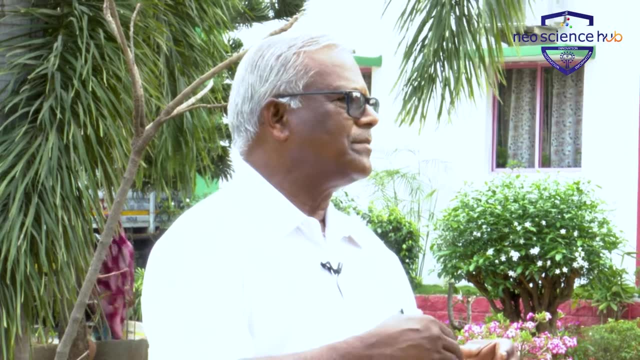 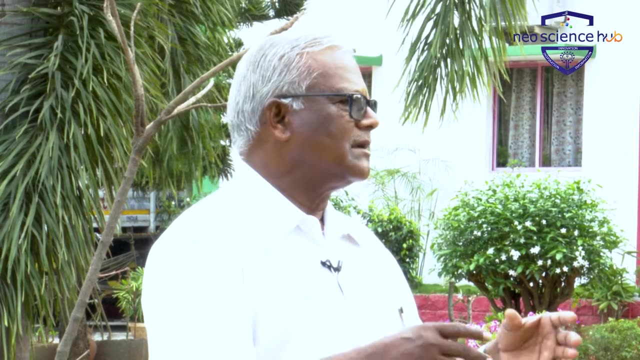 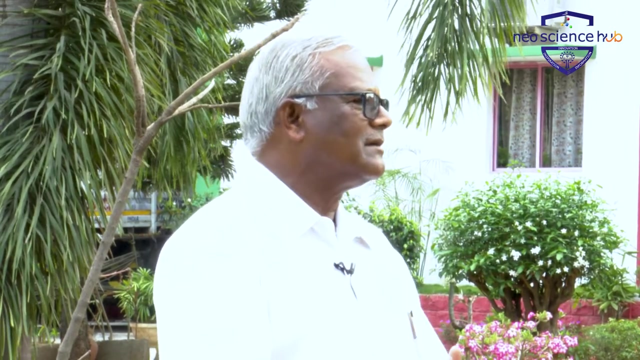 Ok. And they interact with DNA and other vital structures of bacteria or pests And ultimately the pest multiplication. I mean the pest will die with a higher dose, Ok. And bacteria, they may be present but they are inactivated, Ok, See further. while multiplying they finally die. 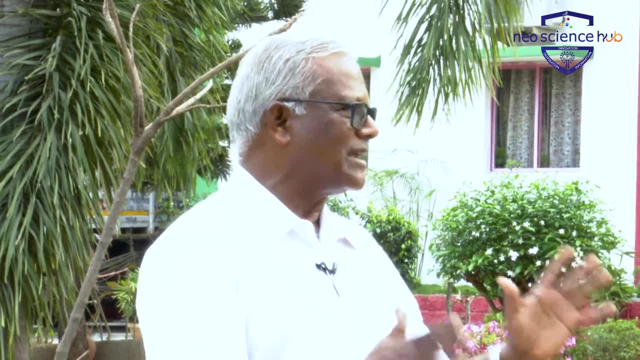 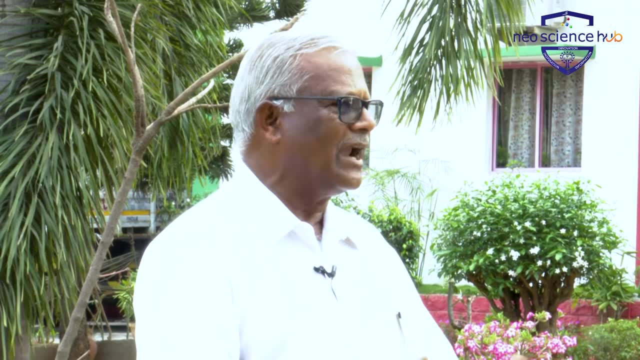 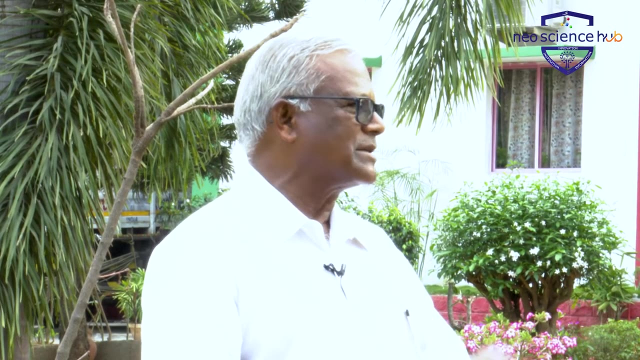 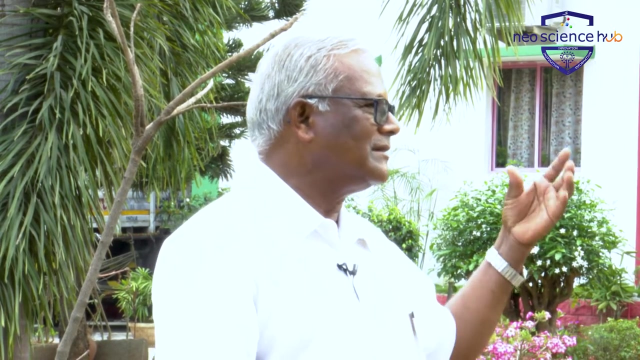 Ok, See, in effect, your food is safe from the pest Pest. how it pest in agro products, especially because of handling and birds droppings. See, invariably pests are present, Pest over are present. These always when find the suitable weather, like humidity, heat, they hatch and larvae are formed. 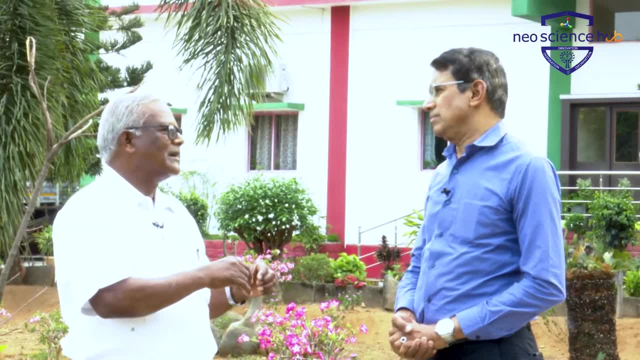 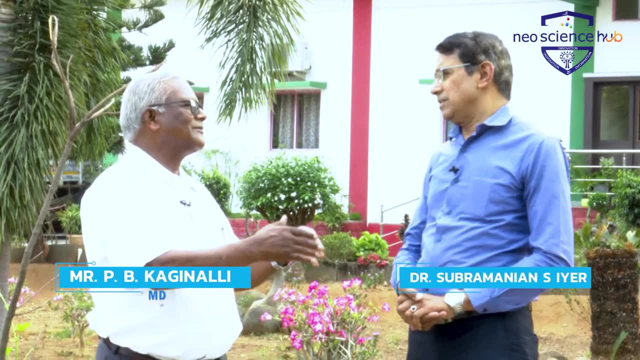 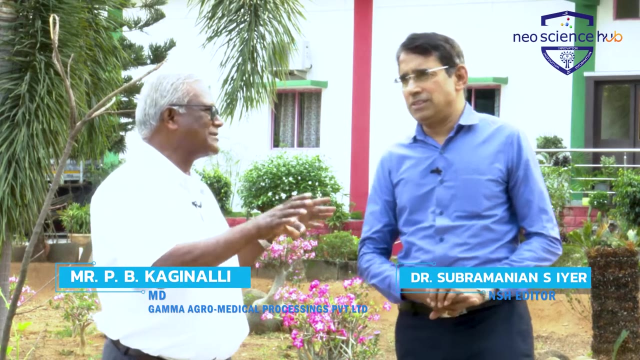 These larvae start feeding on the product And they are moisture, they create moisture. That moisture creates fungus. Very nice, See. ultimately, food gets spoiled. Super, super. See, this is the genesis of, I mean, spoilage of food. Very nice. 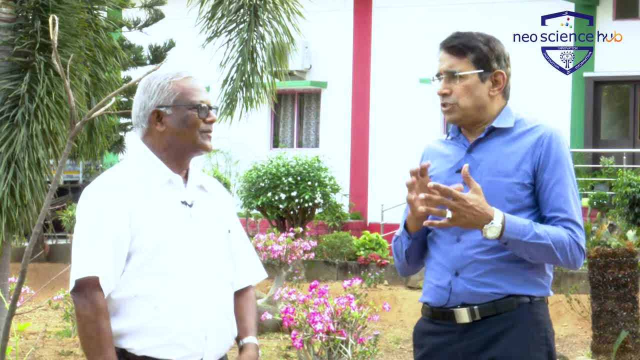 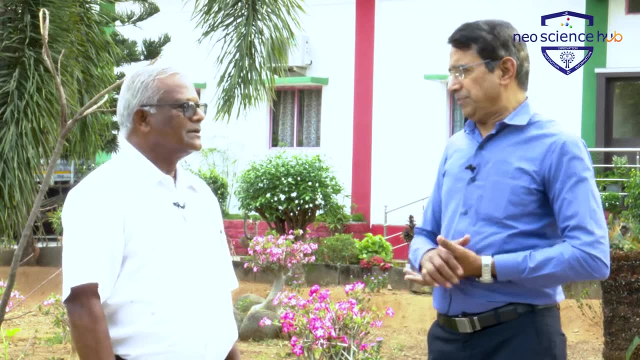 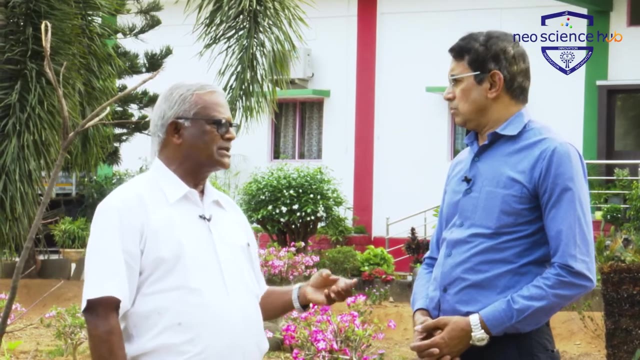 Very nicely explained. Yeah, Talking of food, which, what are different types of food which is getting gamma radiated and is it being exported? Yeah, yeah, Yeah. See, at present we are treating chilli powder in major volume and herbal powders and extracts. 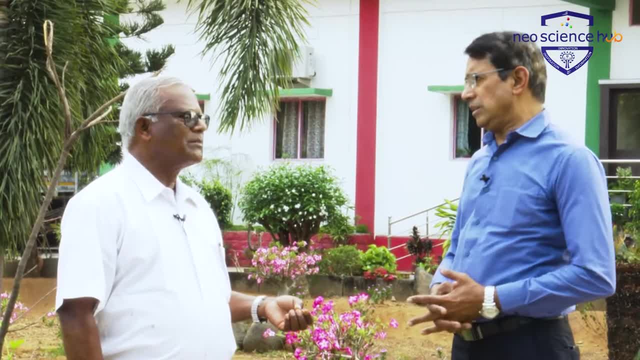 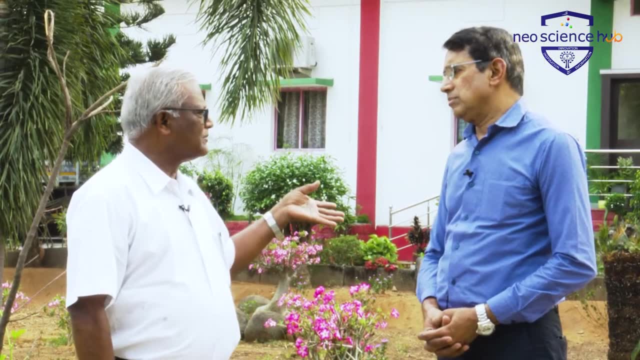 That is because chilli has lot of moisture. because of that, Not moisture, Moisture should not be there. for chilli powder to be there to be treated, Ok, Ok, For me, I mean, harvesting techniques are very crude, Sure. 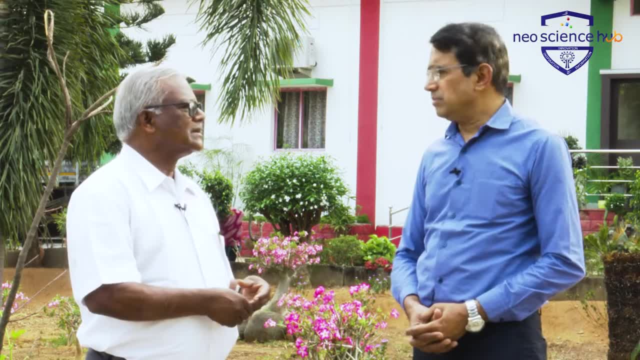 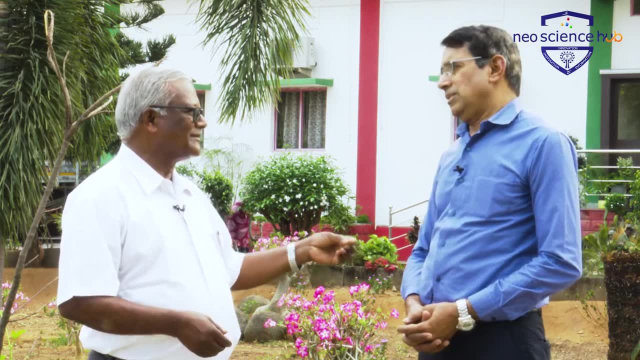 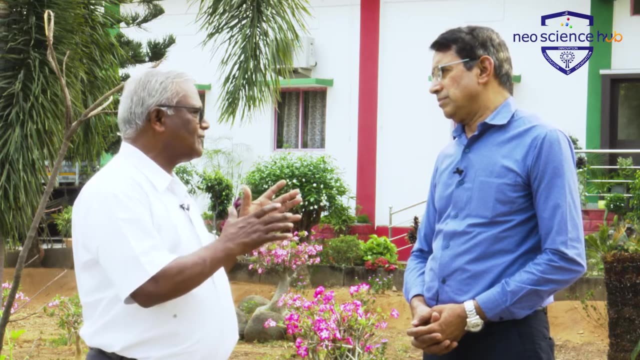 See, invariably they have pest in them, Correct? See, even though it is chilli powder, pest will emerge. Ok, Over, are present, Ok, During crushing this thing, in processing, Correct. And finally, when you just, if you do not treat it and just export during the sea transit. 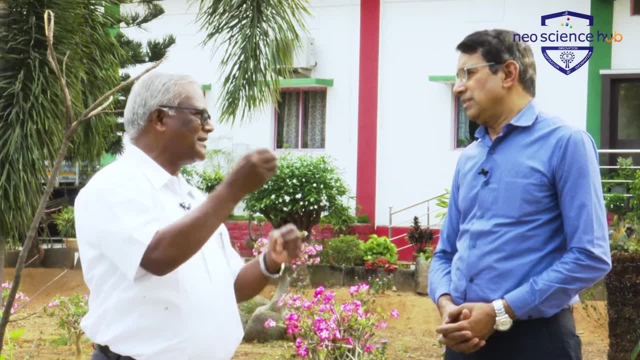 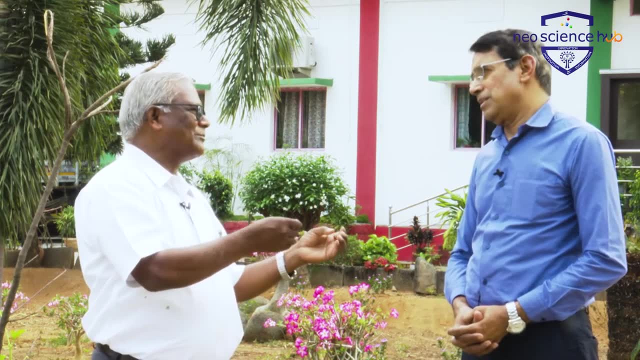 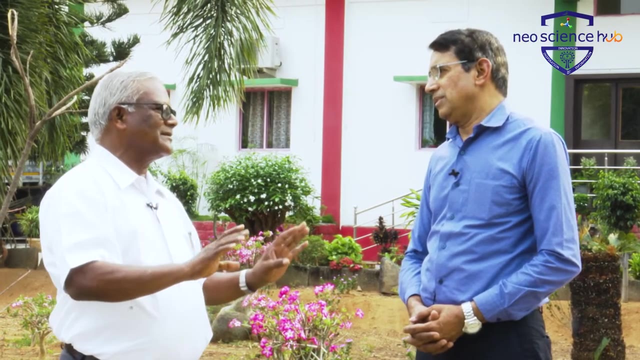 see, because of humidity and heat, by the time the deep destination they may, I mean hatch the oas are hatched into larvae and you will ultimately get the pest there. Ok, See, it would be rejected. Ok, The Europe and American people, they have health conscience and they are very concerned. about any pest and microbes present in that. So that is adding to one more question: What are the norms of western countries in accepting gamma irradiated products? Is there any guidelines or something? Some countries really they have. America accepts irradiated food. 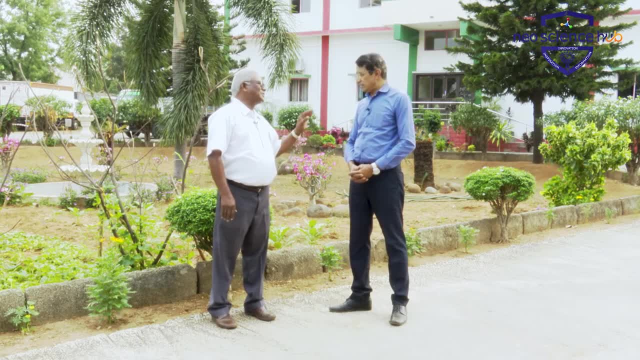 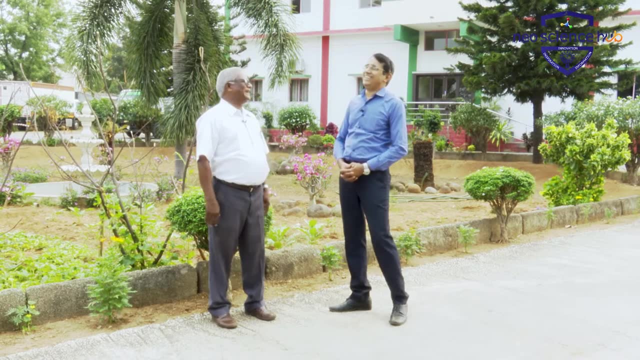 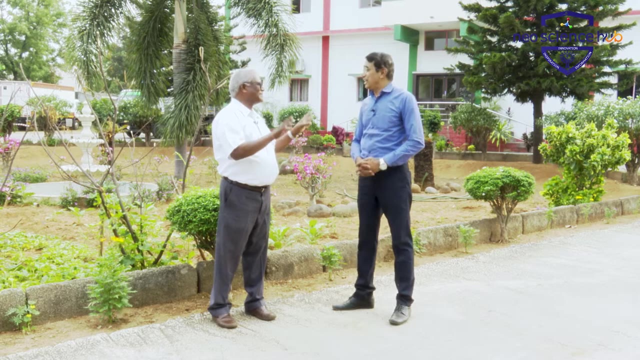 Netherlands accepts, But Germany will not. Ok, And European also has some restrictions. Ok, But dog food they accept. Ok, Dog food is mandatory to be treated by gamma radiation. That is the only item universally accepted, Oh, accepted, For gamma radiation. 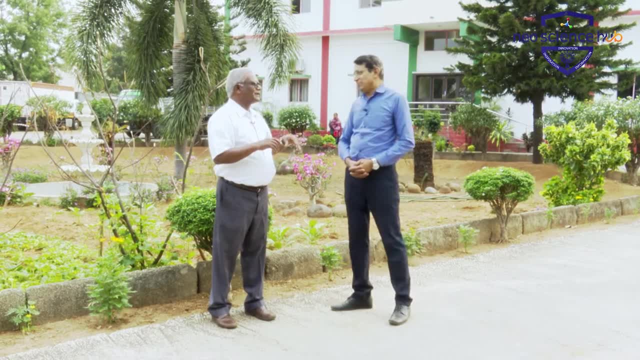 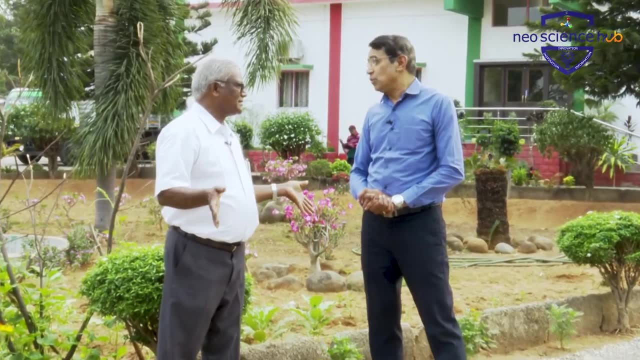 Oh my god, Ok, See, problem is that dog food in our country is, I mean, processed by avatar, rejects Ok, Like ear, Yeah, And this, Ok, I mean trachea, lungs, oesophagus, Ok. 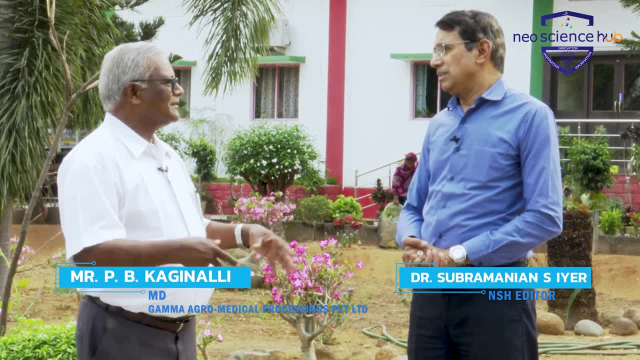 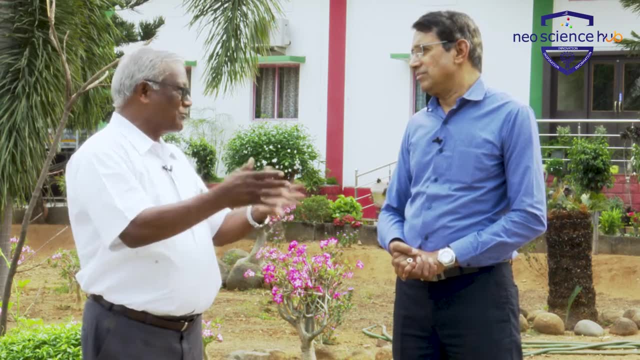 And the intestine- Ok, All these things and bones are also processed. Ok, See, these are all waste. I mean, if you want to, I mean dispose, Ok, Ok. It is the greatest hazard in our country, Ok, Ok. 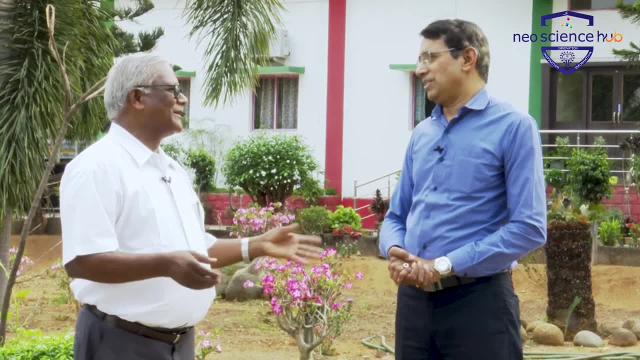 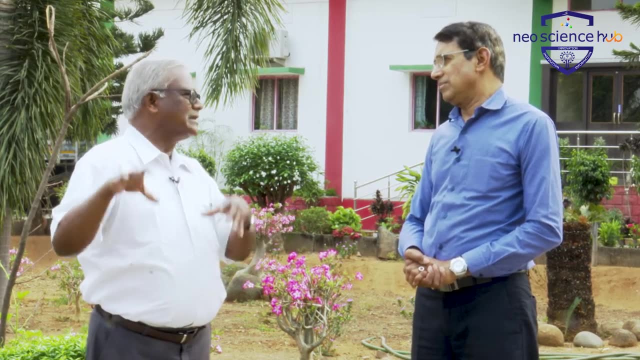 See, the bone is gamma, radiation is a bone. for that I know. Ok, Because they are sun drying. Abundant sunshine, is there? Correct? They can sun dry, Otherwise it is uneconomical. See, they sun dry it and finally little bit of heat, then pack it and send it over here. And invariably this product contains pathogens, parasites and pathogens, See, and more so of this thing called Ecoli Salmonella, which are cause of Microbiology Epidemics Say. that is why they, and more so, why they, want it to be treated by gamma radiation is. 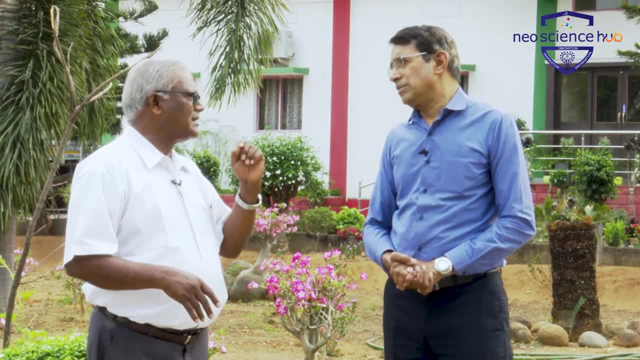 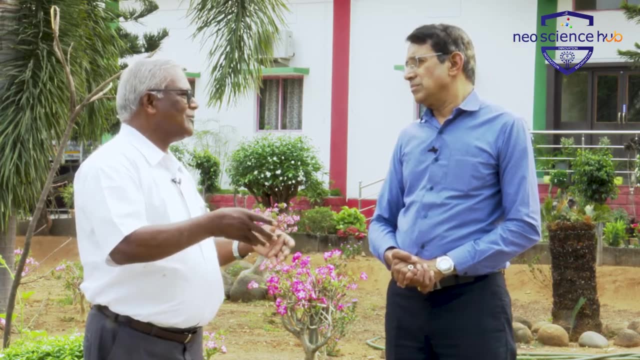 they are very intimate with animals. Ok, They lick. Ok, Himself they lick, and the animal also licks them. Ok, They kiss. Yeah, They have a process. Whatever food it eats, if it is contaminated with Ecoli or Salmonella, it is transferred. 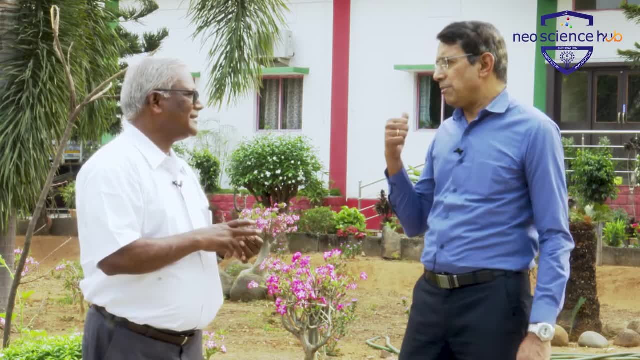 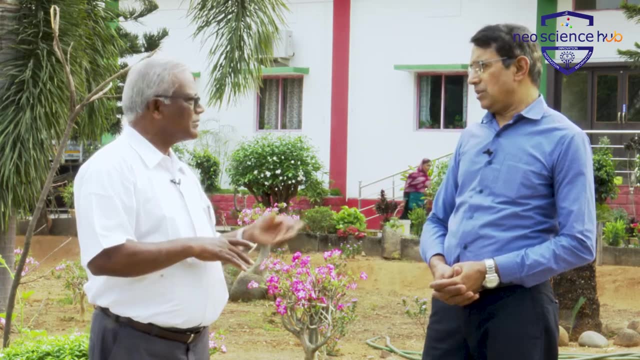 to humans? Talking of Salmonella, are you also gamma radiating eggs in all Egg products? Yeah, Egg powder we were doing Ok, But not much. Ok, Egg powder we can do, Ok, There is no issue. So how do you know that this sterilization is sufficient for this? 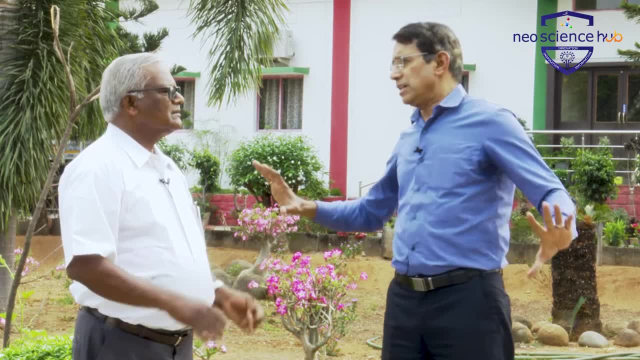 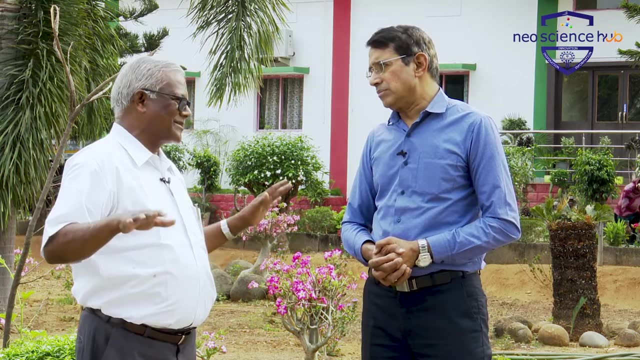 Is there any calculation based or is there a standard formula? No, there are. See, there are lot of works have been done. Ok, For almost 40 years. Ok, This technology was dropped for certain reasons. Ok, And unscientific reasons. 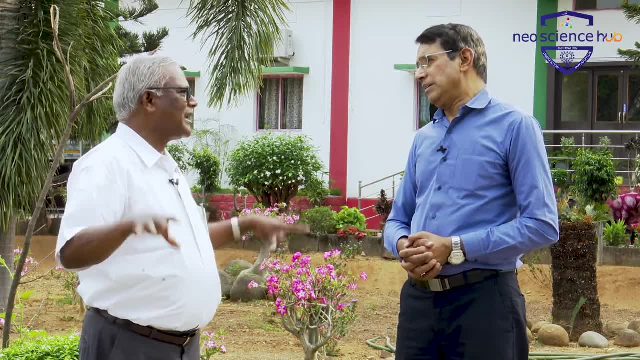 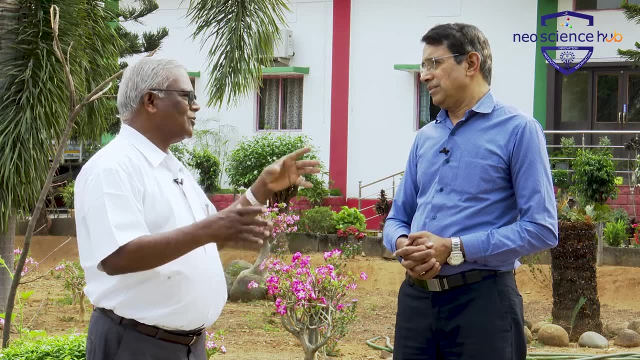 Ok, So then they are realized, and cobalt is not a radiation which is to going to be remain analyze nuclear bomb. I know, I know It is in a gas form or water form. Yeah, It is a sealed isotope, Correct? 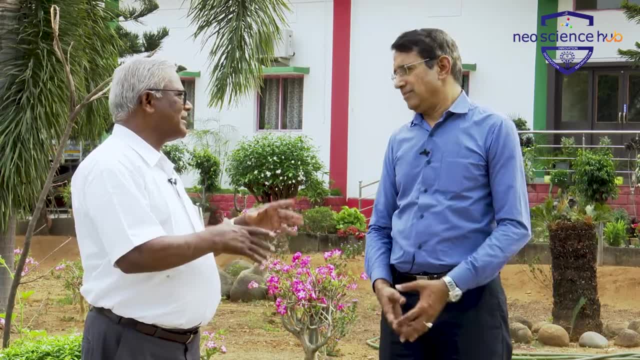 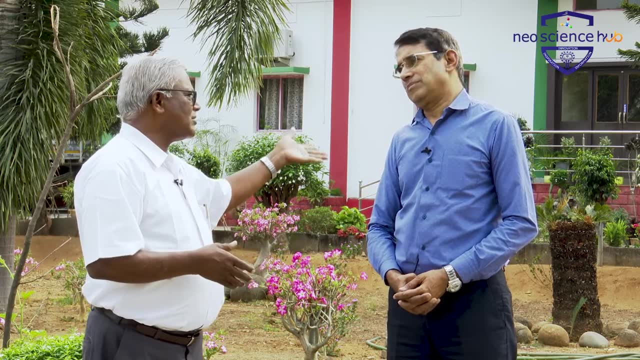 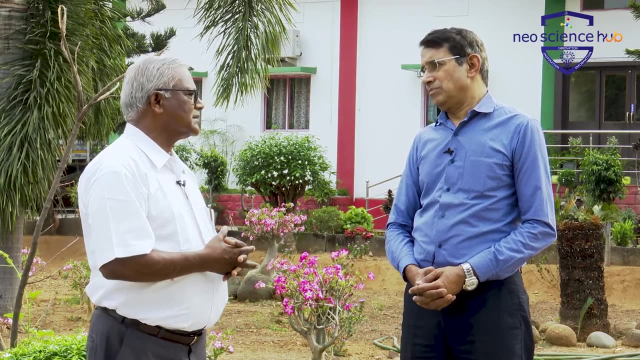 And which can never contaminate anything unless it is properly managed. Managed, So, So, So, So, Yes, Managed, See, there is no fear of contamination as long as we take care of it properly, Ok, And that does not leave any radioactivity remnant, these things at all. 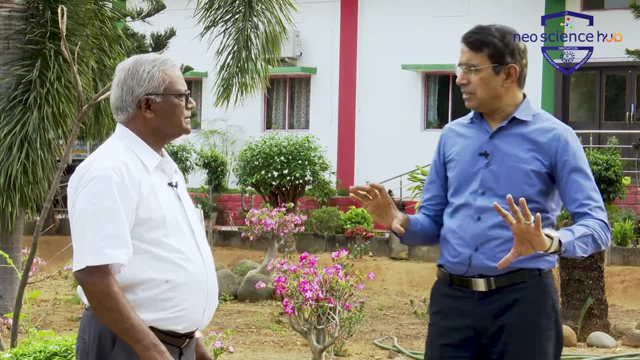 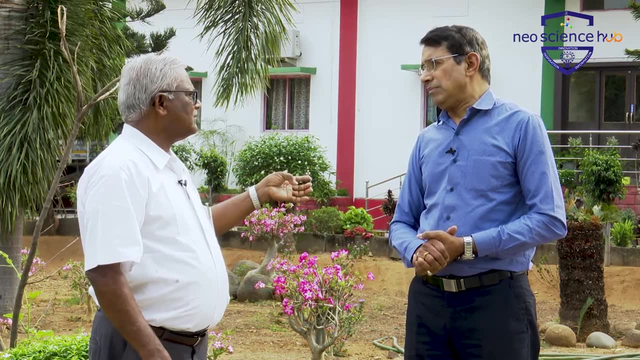 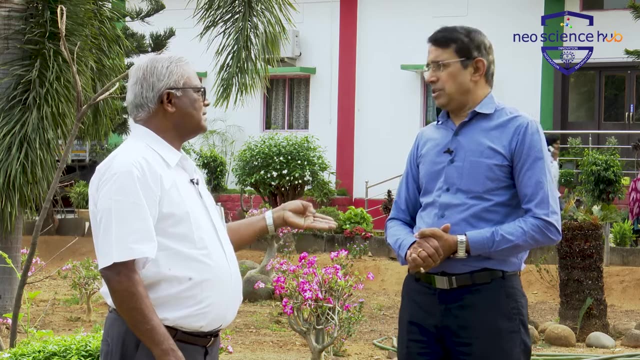 So you mean you have a set of guidelines for each product? Yeah, For which you Medical Chili powder and all. See, depending on the criteria, there are certain units of energy, Exposure, Exposure, Correct. Those, Yes, Those to be delivered to the product. 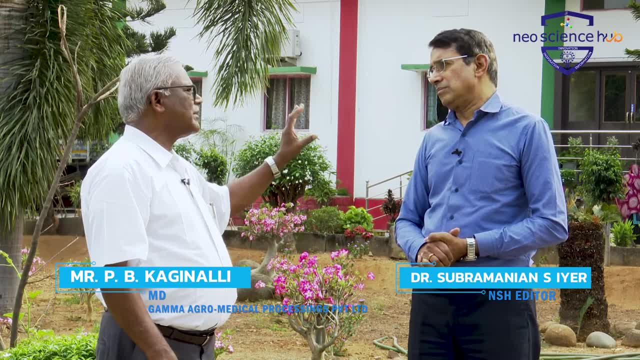 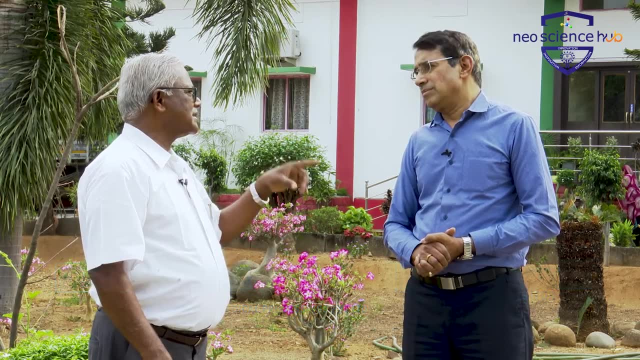 Ok, Ok, See, normally what we are treating is here is about 8.5 kilo gray. Kilo gray: Kilo gray: One gray is unit of energy, of one joule of energy in one kg of product. Ok, Ok. 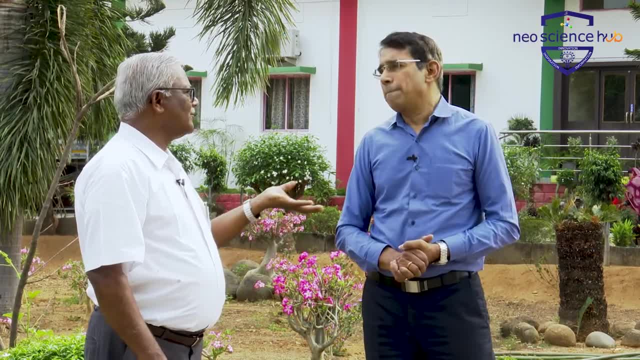 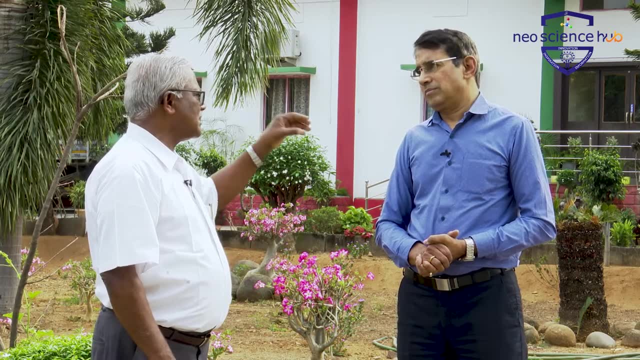 Ok, One joule in one kg of product. Ok, Like that kilo gray, We work in kilo gray. Ok, 8.5 kilo gray for food product and this pet food, chili powder. any food product for that. 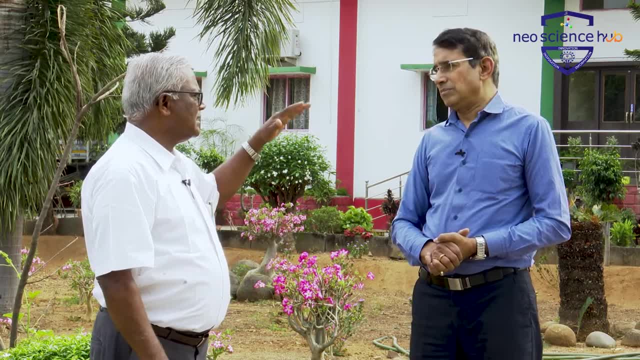 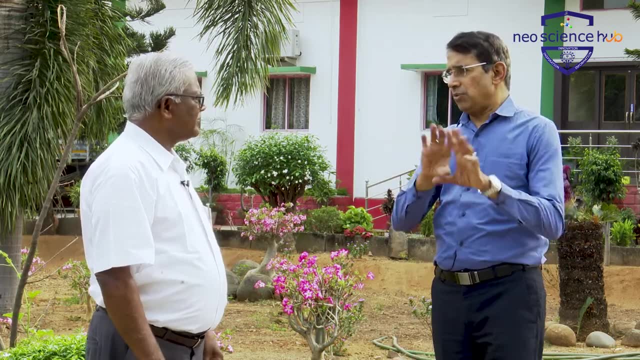 matter is good enough. It removes all salmonella, E coli pests and most of the bacteria, So you give a certificate in the end after that. Yeah, Exposure certificate, Exposure certificate. Yes, This product has been irradiated with a dose of this much. 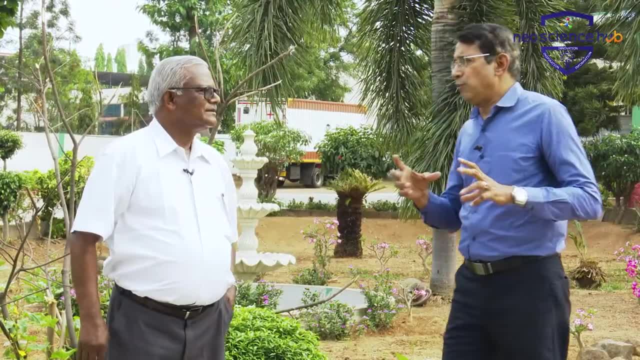 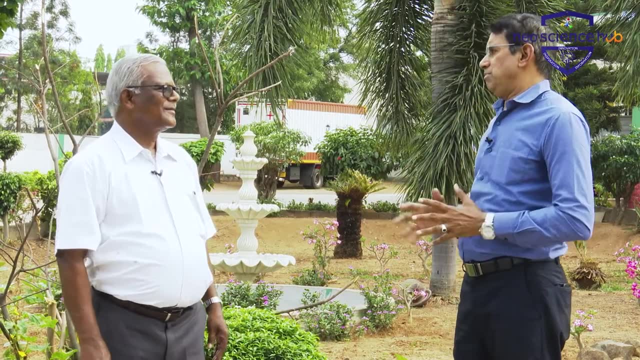 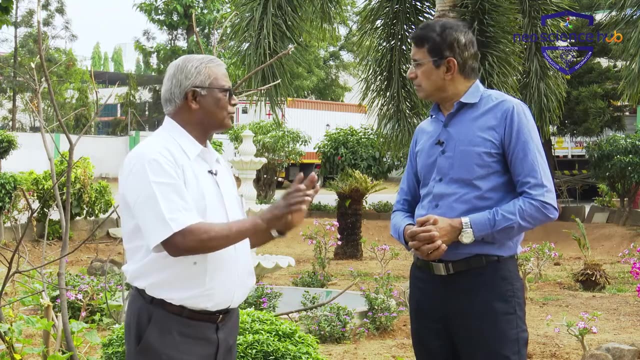 Ok, Ok, So we issue a certificate. Ok, I am forced to ask one more question. Ok, What is the shelf life Post variation? How long will a product be free of microbials? There is a certain shelf life of natural, shelf life of product. Correct. After certain period it loses its potential or vitamins or whatever. it is Absolutely See after treatment. as long as you don't open the package, Ok, Ok, The product remains safe. Even I have preserved for 5 years Super. 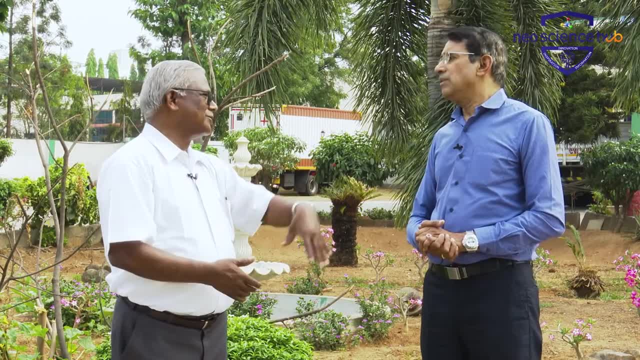 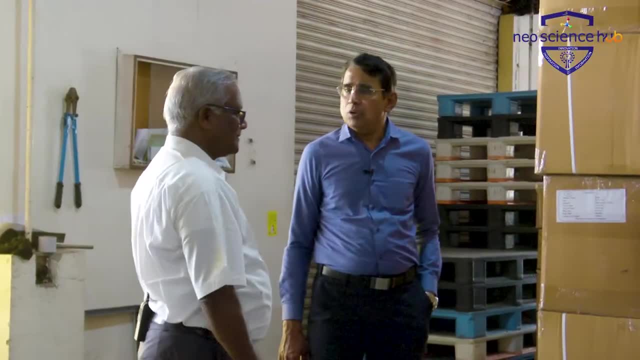 Nothing had happened. Super, As per physical things are concerned, Internal things need to be studied, Of course. Of course, The shelf life we can give Unopened. Unopened The dog food. Oh ok, See, it is a tripe we call it. 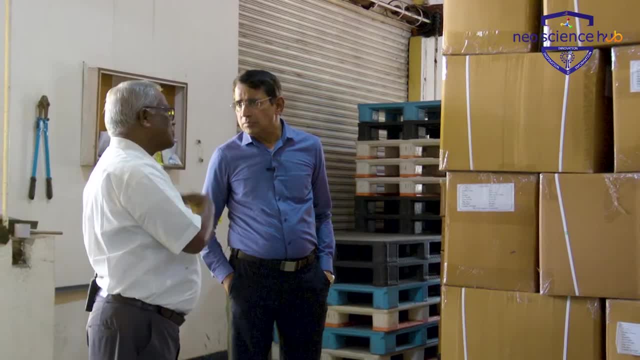 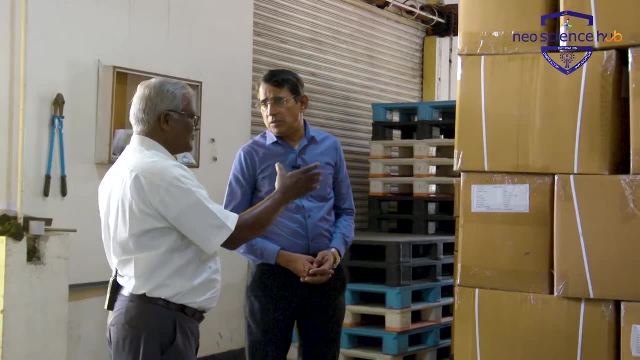 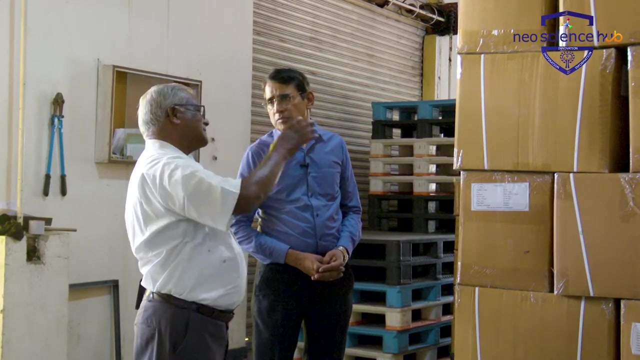 Ok See, it is a trachea portion. See from this down. Ok, That is not fit for human consumption. Ok See, that is dried and packed. Ok, And it is for Export. Export, Export only, Export only. 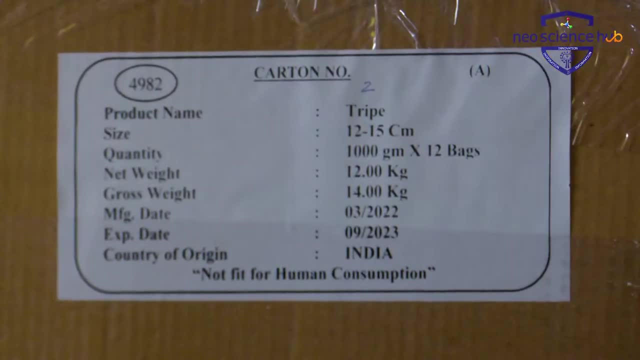 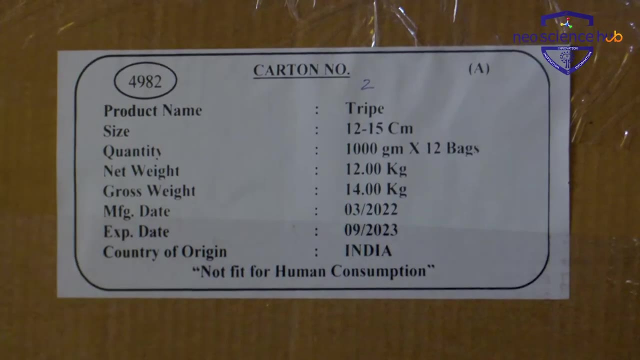 Export only. Ok, Mostly it is Europe and US. When you say trachea, is it dog trachea? is it Dog trachea? Oh, ok, Dog trachea and buffalo Buffalo- Mostly buffalo, Not dog Dog food. 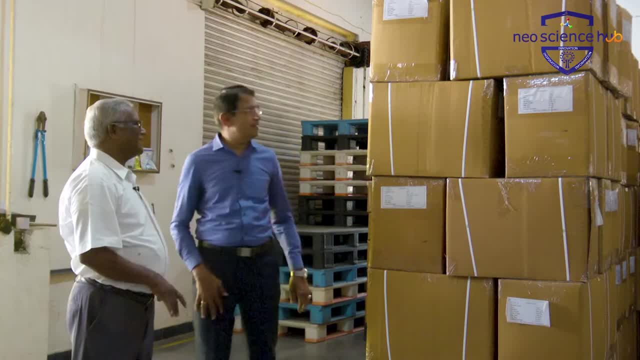 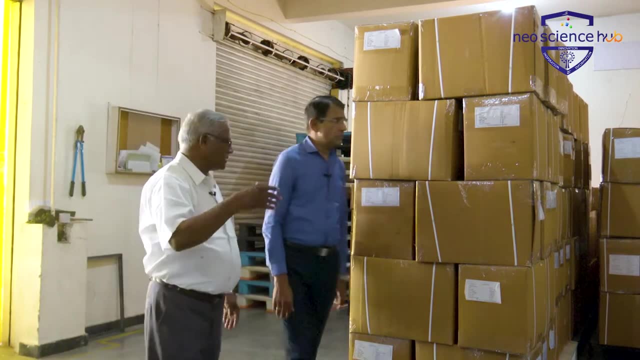 It is a buffalo meat, Buffalo or foie gras. Yeah Yeah, Buffalo foie gras. Yeah, Oh, ok, Ok, Ok, So this is made in India, is it? It is here, only There are two plants. One plant is there in Aurangabad. 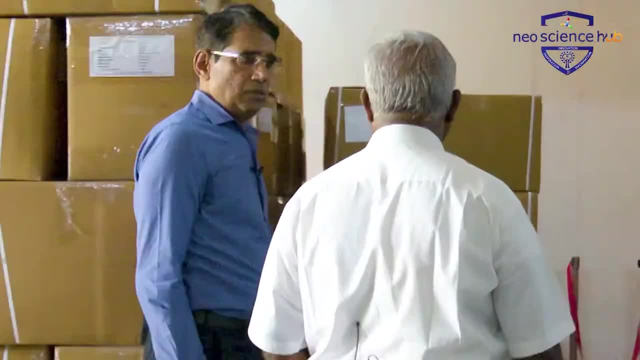 Another plant in Jeherabad. Ok, In north also they have. Thank you, Mr Karim Ali. That was an excellent tour of your facility, Really good tour. Just trying to ask you one more thing: How many such facilities are there in India? 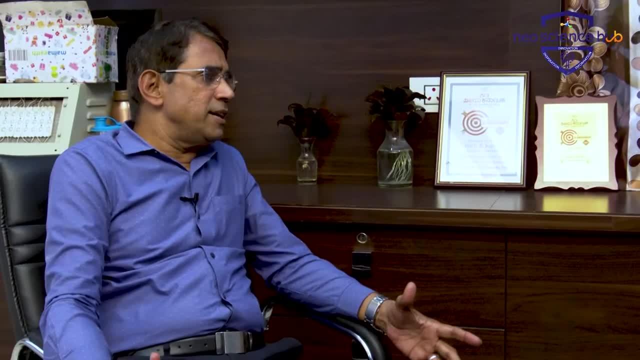 There are 14 facilities in operation at present. A few more are under implementation. Most of them are concentrated in Bombay. There are 5 facilities in Bombay itself. Ok, Ok, See other things are being done. Ok, Ok, Ok. 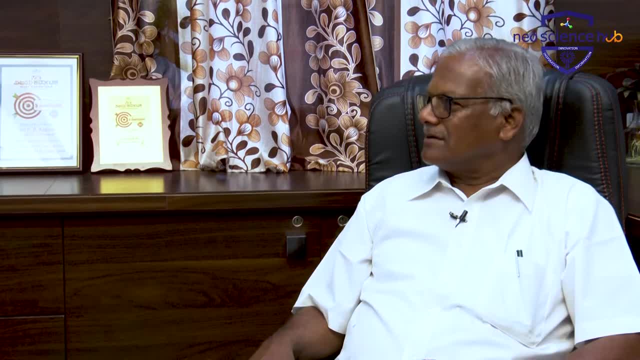 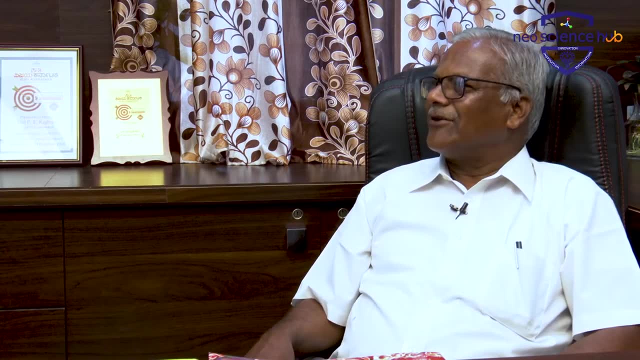 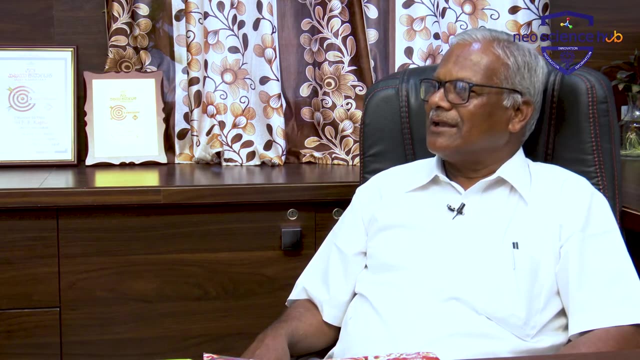 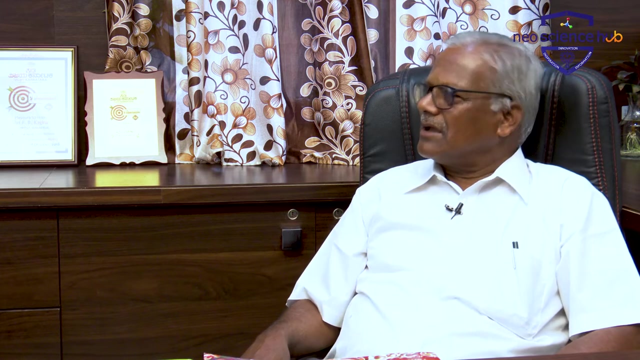 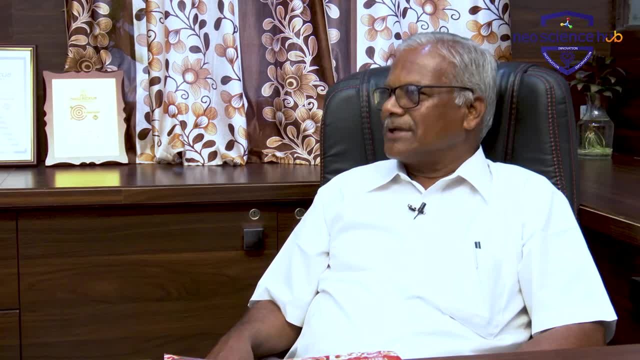 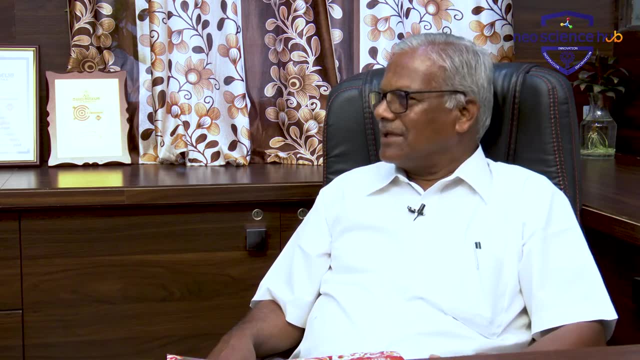 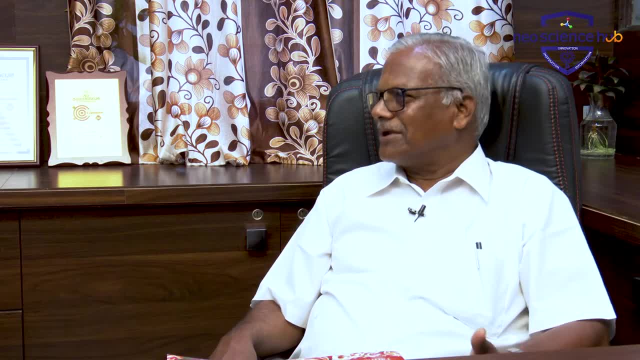 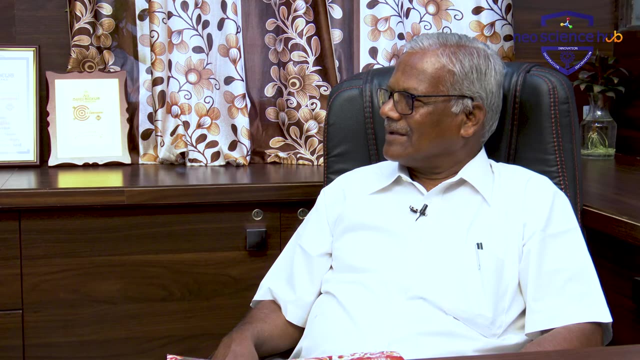 In Bangalore. there is one In Kerala. we are getting material from Kerala also. There is no facility in Kerala. So this is the scenario in the country. Sir, one more thing which I am forced to ask you is: some people have this opinion that any variation is detrimental to health.